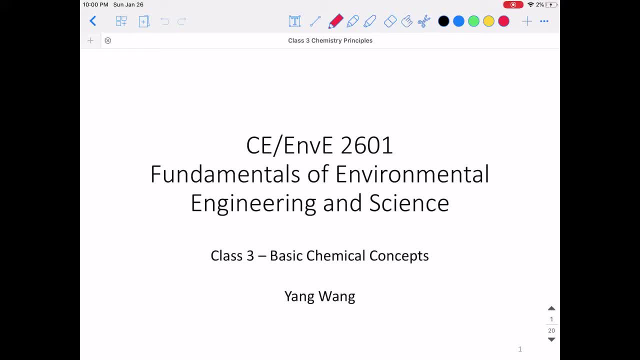 Okay, hello everyone. So let's continue our lecture on the fundamentals of environmental engineering, And so this class we're going to continue reviewing some basic chemical concepts so that we can apply these concepts into water treatment and wastewater treatment. So before we do that, let's do a quick recap. 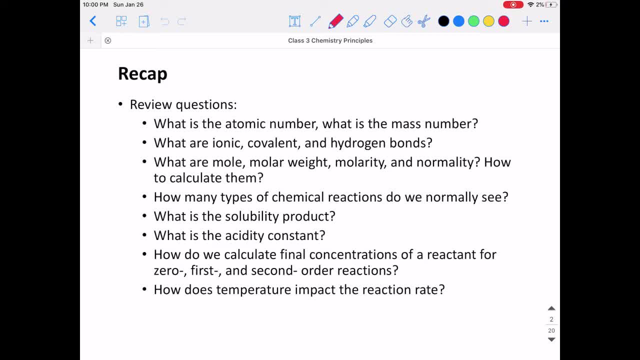 of what we have learned in our last class. In our last class, we mainly went through quite many basic chemical concepts right, For example, including what is atomic number, what is the mass number. so this is related to the structure of the elements. And also we learned what are ionic, covalent and 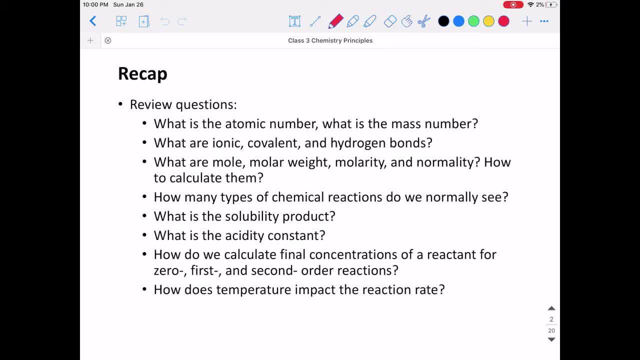 hydrogen bonds, and these are related with the forces being applied onto the ions or the elements, And also what are the mole, molar weight, molarity and normality. So in this class we're going to learn more about the molarity and normality in the water and wastewater. 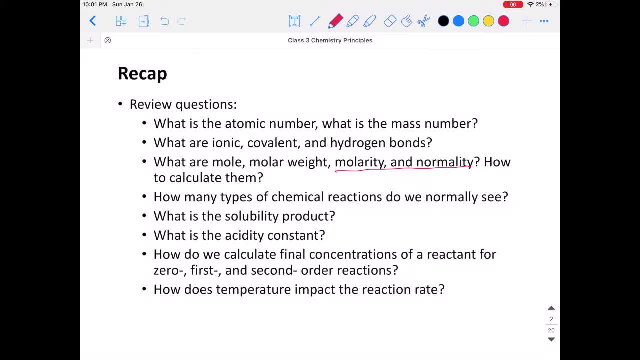 treatment And also how to calculate them. Furthermore, we learned: how many types of chemical reactions do we normally see? For example, we have the redox, basically the reduction of oxidation reactions. Right, We also have the precipitation reactions. And also: what is a solubility product? What is the acidity constant? So, 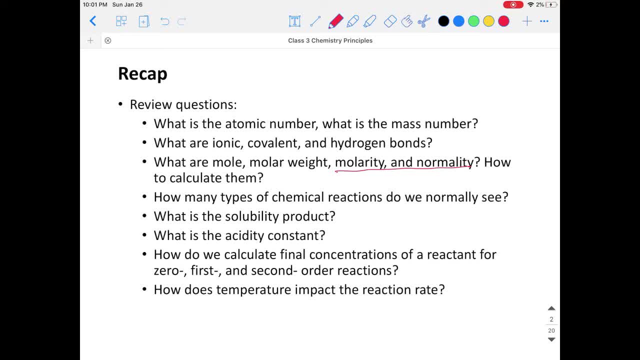 how do we calculate the finite mercury ages in water? So what is the? just the concentrations of a reactant for zero first and second order reactions, right, And also what is the temperature influence onto the reaction rate. So we have some empirical equations that can consider the temperature influence onto 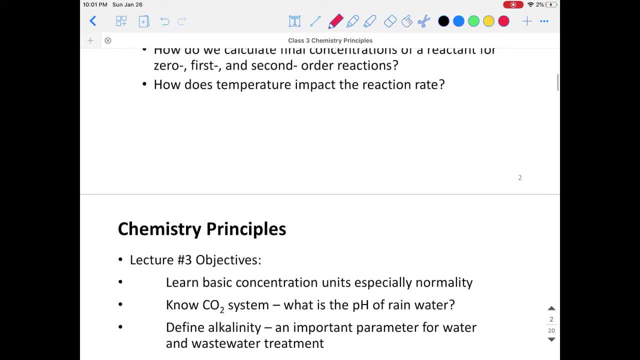 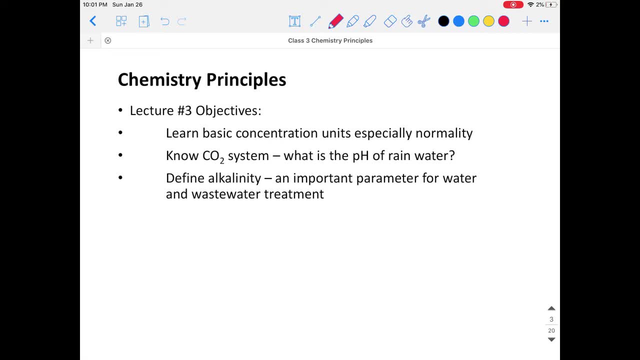 certain reaction rates right. So in this class we're going to learn more of the basic concepts that can be used in environmental engineering. So we're going to learn basic concentration units and especially the normality. so this is a quite new concept that we're going to use And also we want to know the 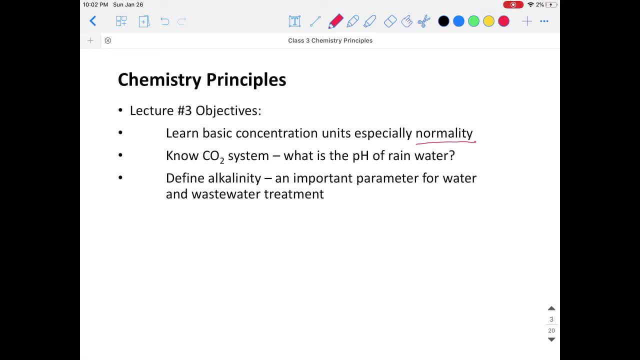 carbon dioxide system. What is the pH of rainwater? Because there are a series of dissociation reactions that will determine how the hydrogen ions are being released in water And also we want to define the pH of the hydrogen ions And also we want to define the pH of the. 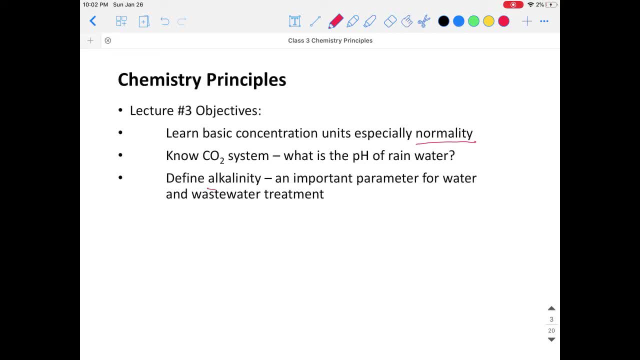 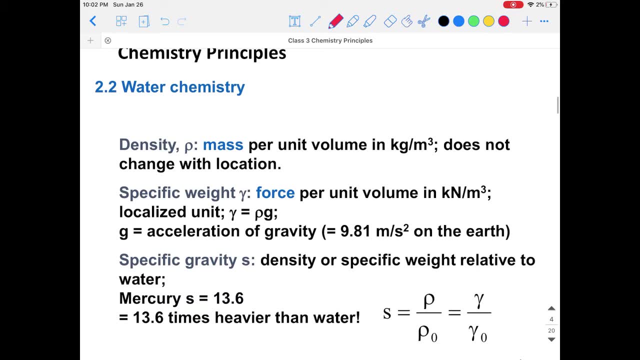 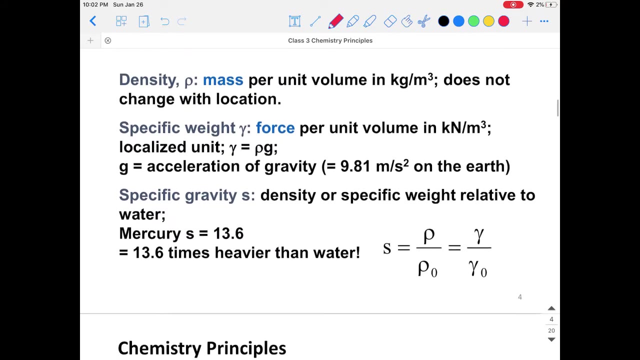 hydrogen ions, And also we want to define the alkalinity, and alkalinity is actually a very important parameter for the water and wastewater treatment. So first we want to learn some basic concepts that can be used in water chemistry, And here I'm going to quickly go through some definitions that we used before, For 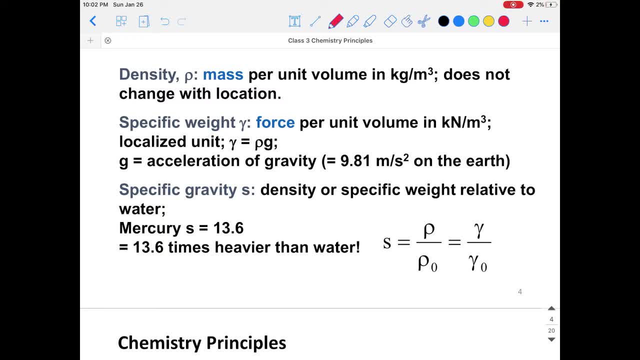 example, the density. we know that quite well. Actually, the density is a mass per unit volume in kilogram per meter cubed. So it does not change with the location, right, It doesn't matter whether we measure it at the surface of the Earth or in the space station. So there's. 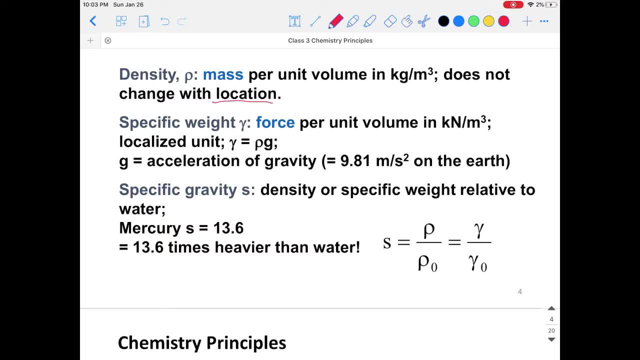 another definition, called the specific weight, and the specific weight is related to with the gravity. It's basically the force per unit volume and that can be represented in kilonewtons per meter cubed. So basically the specific weight or gamma can be. 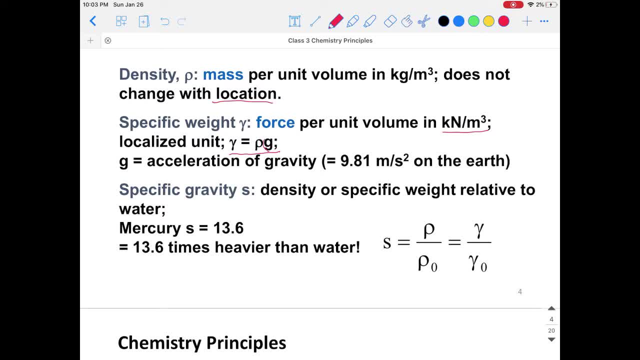 calculated by rho multiplied by g, where g is the gravity and the gravity can be different at different locations. right, the higher the- basically higher the in the sky, then the lower the gravity or the acceleration of the gravity. right, so there's another concept called the specific gravity. we normally use s as 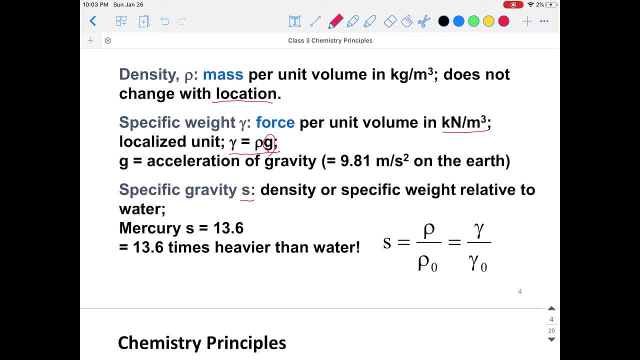 the parameter or as a symbol. so that is the density or specific weight relative to water. so, for example, the mercury have a density of 13.6 grams per centimeter cube, so that's a 13.6 times compared to the 30 point 13.6 times of the water. 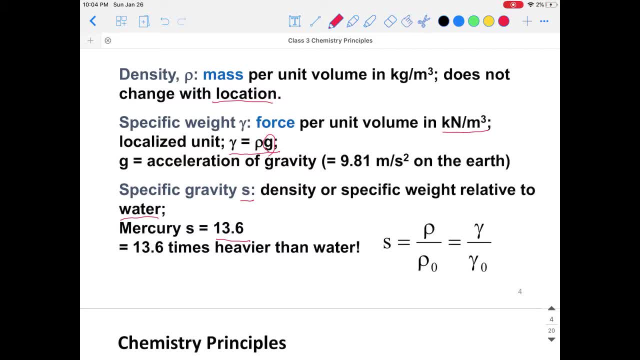 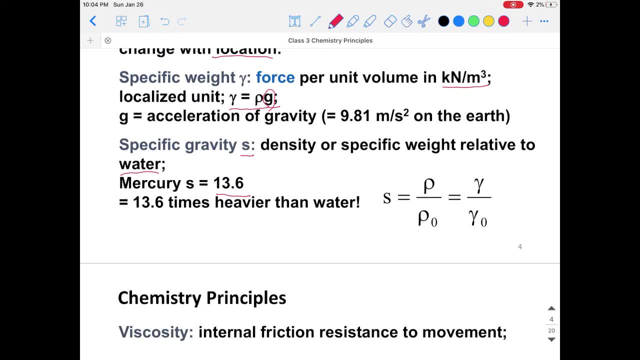 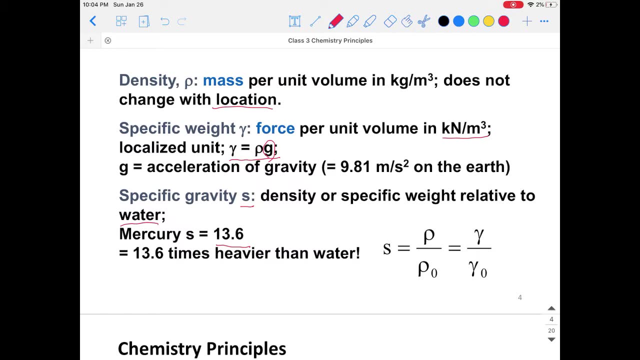 density. so under this situation, the specific gravity for mercury is going to be 13.6, which also means that is 13.6 times heavier than water, and based on these definitions, we can know that specific gravity can be also represented by the ratio of the density of certain object or certain species. 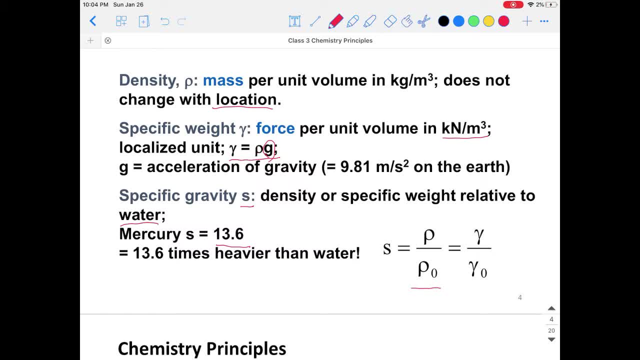 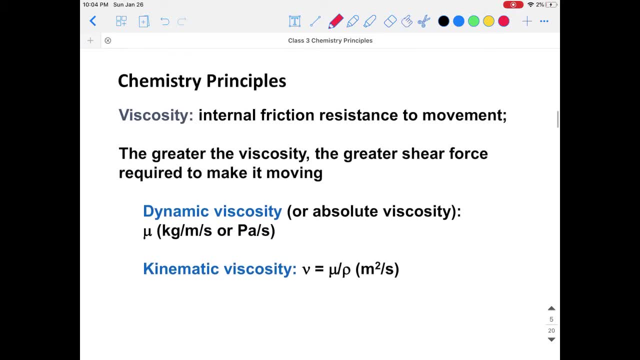 over the density of water or the specific weight of certain species over the specific weight of water. so in water chemistry we're also going to use the viscosity of the water. so the viscosity is defined as the internal fraction resistance of the water and the density of the water. so the density of the water is. 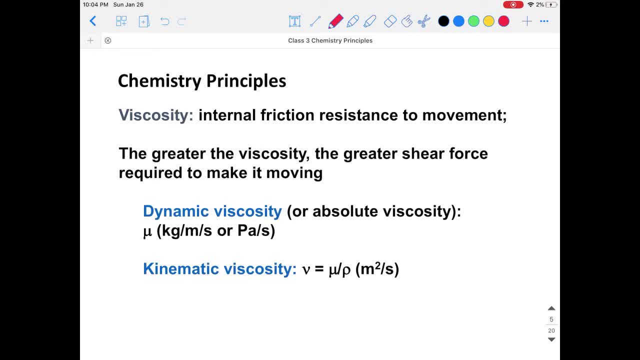 the resistance to the movement. so basically, the higher the viscosity then the more difficult it is to move certain liquid or to cause the movement to this liquid. so basically, the greater the viscosity, the greater the sheath force that it will going to require to make it move. 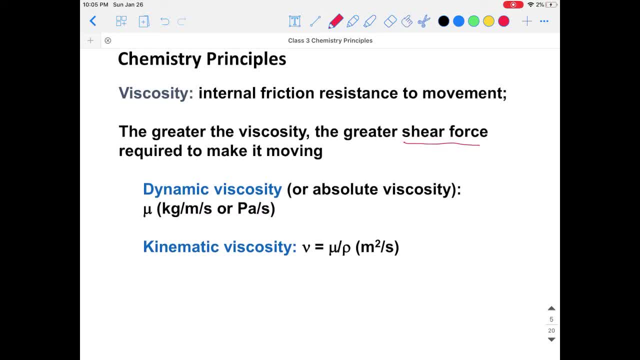 and in terms of the parameters that we can use to quantify the viscosity, we can either use dynamic viscosity or that's also called absolute viscosity. we normally use Mu, and Mu is going to have a unit of kilogram per metre per second or posca per second. 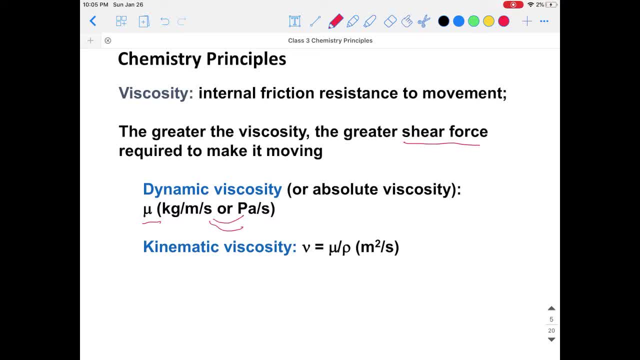 so basically these two units are the same and we can also define a kinematic viscosity and the kinematic viscosity includes the influence of the density for the liquid or gas species. so that can be calculated by mu equal to mu divided 4 star mu and mu divided 22 stars: 35주. 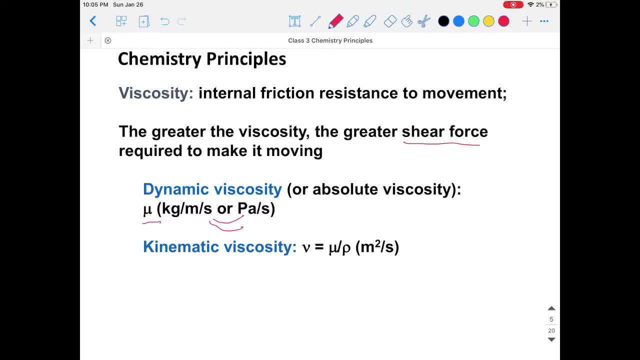 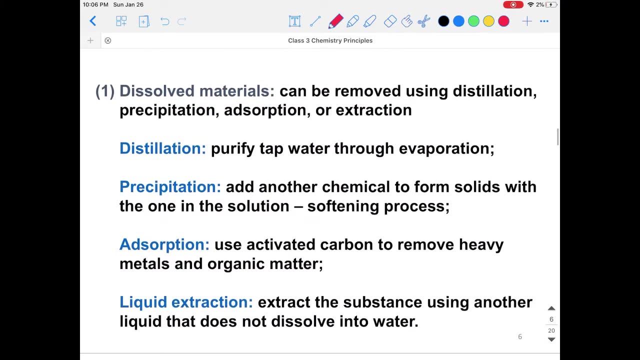 plus Mgu, plus CuCu, foriest plant temperature or normalد 지난쳐ilar성 by rho and based on that, if we plug in the density of the plug in the unit of density we're going to have the unit of meter squared per second. so in water, 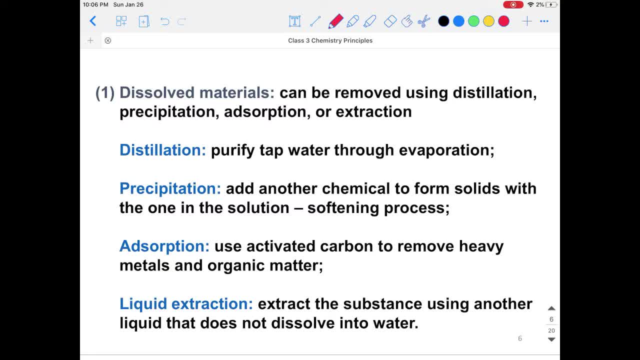 chemistry and we're also going to deal with the basic mixture of species that can be interact, interacting with the water. so for these extra species, they can exist in different states, for example. for example, they can exist in the dissolved materials, which means that they can be removed using distillation. 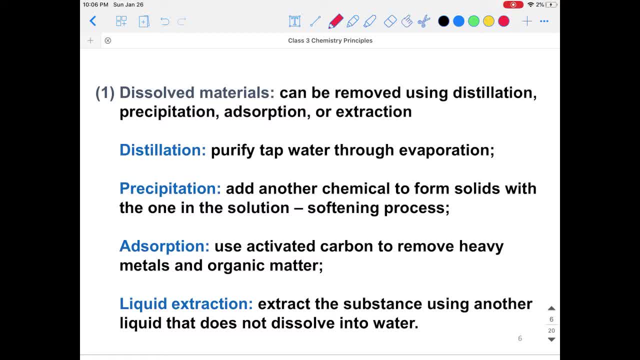 precipitation, absorption or extraction. so distillation means the, the purifier, and the purification of the water through evaporation. so basically, we know that if we're having a field trip outside and we need clean water, what we can do is that we can collect the rainwater. 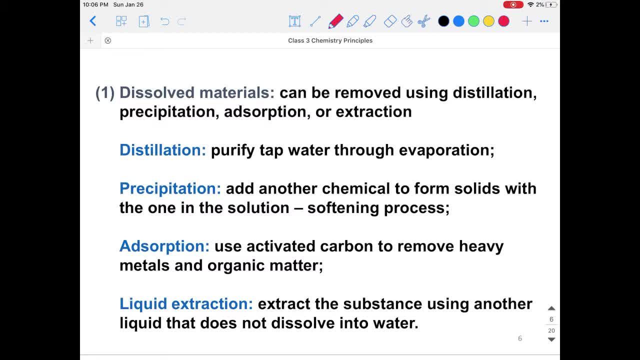 and evaporate them, so further collect them with some devices at top of it, right? so this process is called the distillation, so that will basically evaporate all the water contents into the gas species, into the gas phase, and they can further get condensed and then collected, while the remaining, or the 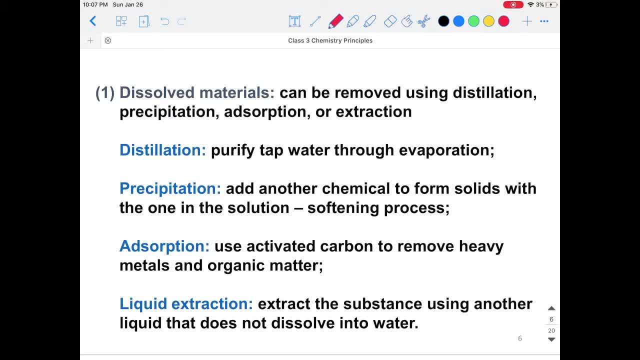 dissolved materials will remain in the solid phase because they cannot be easily evaporated. we can also use the precipitation method, so what that means is that we can add another chemical into the solution and then to form liquids, so basically, these to form, to form solids. so basically, these solids will. 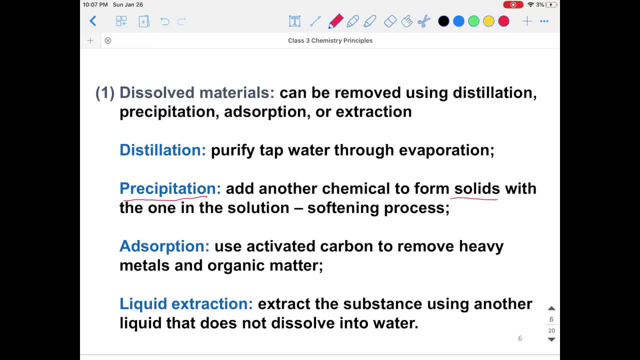 precipitate or settle down within the, within the liquid mixture, and this method is commonly used in the softening process and we're going to learn that in the water treatment we can also use the adsorption. so adsorption means that we can add in extra solids. for example, people can add in sand into water, because the sand can. 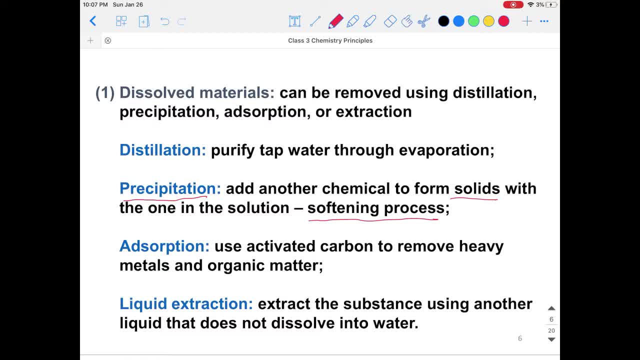 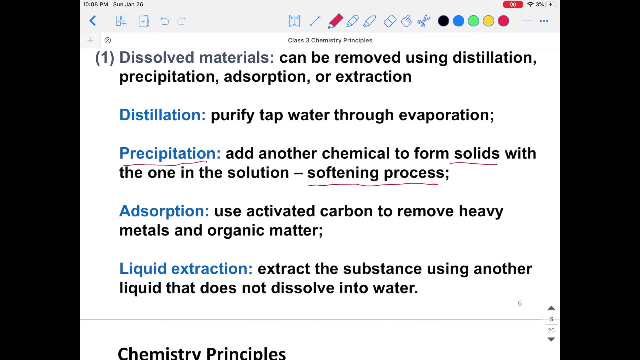 have a relatively larger surface area and these surface areas can adsorb other species from the water. so basically, we can also use the activated carbon and that can remove the heavy metals or organic matter, and we can also use the liquid extraction. so basically that means what that means is that we can extract the substance using another liquid which 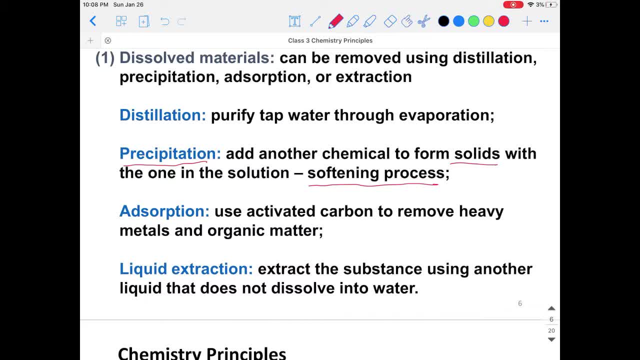 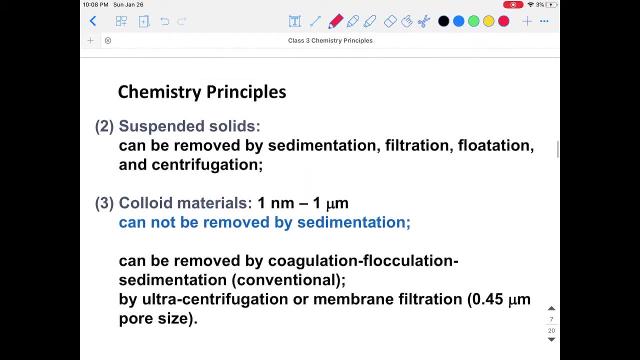 means that these extra species in water probably can better get dissolved into this another substance- substance right? so in this case we can separate the extra species from the water. so these extra species can also exist in the form of suspended solids so they can be removed by sedimentation future. 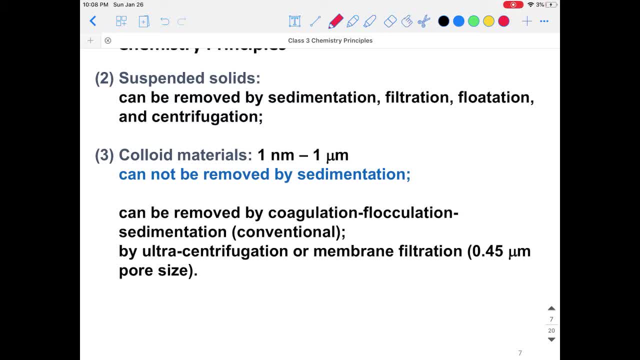 filtration, flotation, centrifugation. So what that means is that we have, if we have larger particles or larger suspended species in the water, then we can just let it still there so that its gravity is going to remove these extra solids. And we can also use the filtration, for example, use the sand. 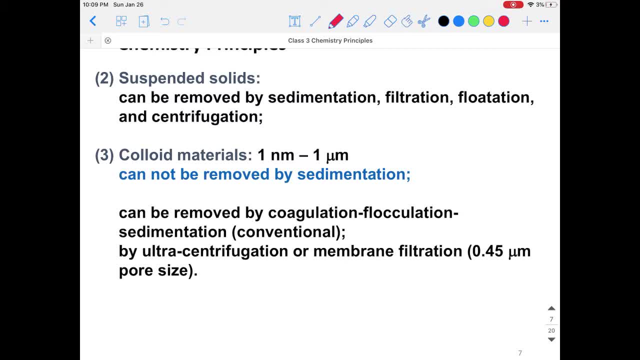 to collect all of these extra solids, right, And we can also use the centrifugation, because if we create a rotational movement, then basically these larger solids will have will need a larger centrifugal force to sustain their rotation if they don't have that extra centrifugal force. 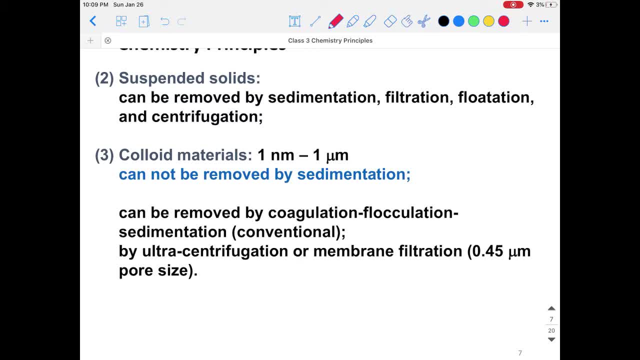 they can be basically get removed from the water or from the liquid phase, And there can also be colloid materials. So what that means is that they are also categorized as solids, But they are in the range of a solid and kind of solid material, And also they can be in the range of 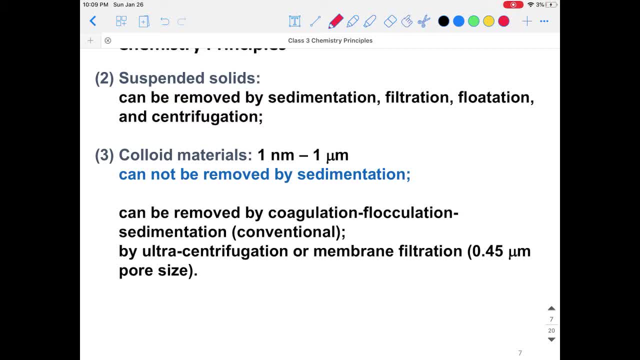 of one nanometer to one micrometer, and they cannot be easily removed by sedimentation because the mass of them or the gravity on these small particles are so small, So it's going to take a very, very long time for them to get removed by sedimentation, right? So under this situation, 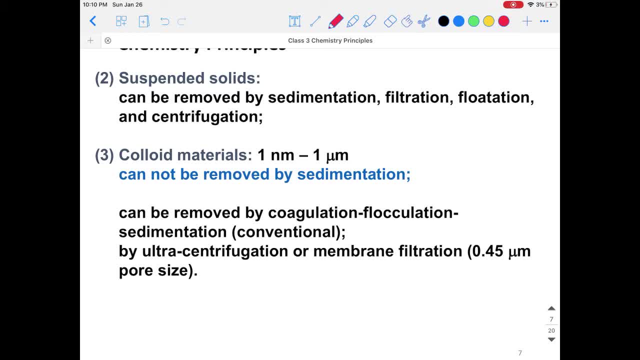 we can use the coagulation, flocculation, sedimentation, So this is a conventional method, And we can also use the ultracentrifugation. So what that means is we can create a very strong rotation movement of the liquid so that we can remove these smaller particles, Or we can just 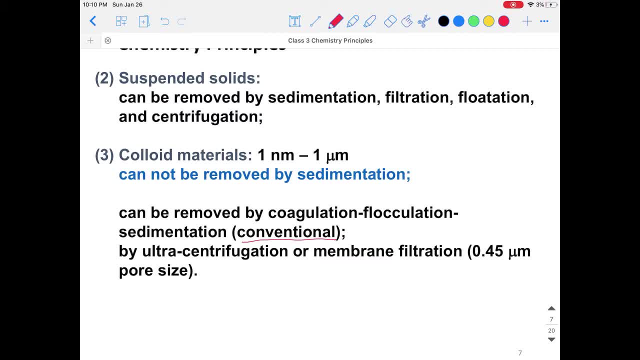 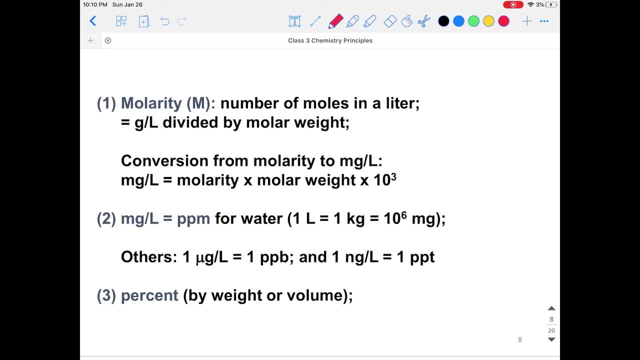 use a membrane filtration to get rid of these particles. So in water chemistry there are also other concepts that we need to know. So, for example, we need to know what is the molarity. So the molarity is typically represented by this capitalized. 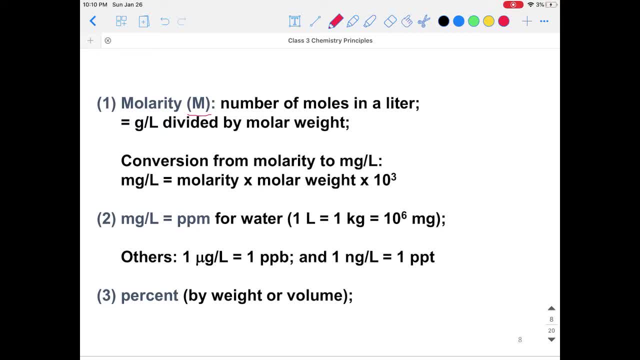 letter M, So that means the number of moles in a liter. For example, if we prepare a solution that's containing sodium chloride- right, we know that its concentration is one mole per liter- then the molarity is going to be one M. Okay, so this is a convention. For example, 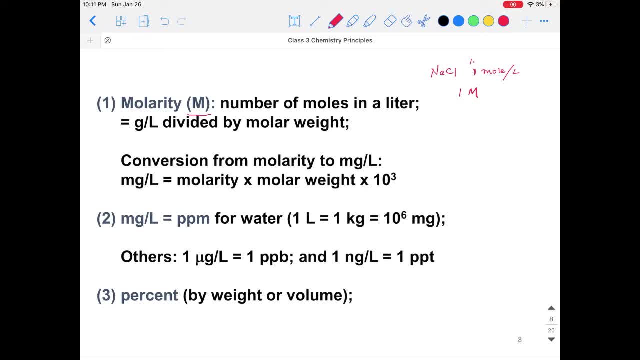 if we decided to prepare another solution of sodium chloride which is containing 1.2 mole per liter, and then that's going to be 1.2 M. So this is the molarity. So after we know the molarity, we can easily convert from these concentrations, from this molarity, into mass. 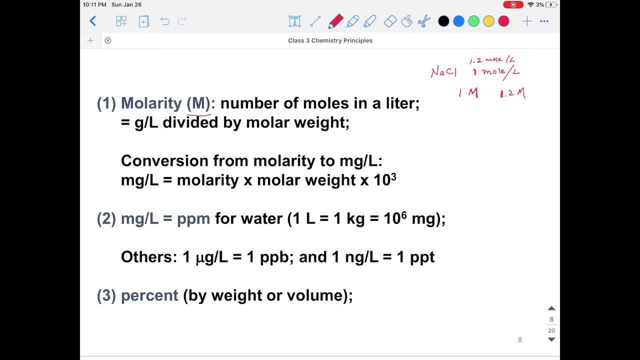 concentration right? So basically we can convert if we know the molarity, and then we can measure or we can multiply the molecular weight of these species to get its mass concentration. And normally for mass concentration we define, we use a unit of 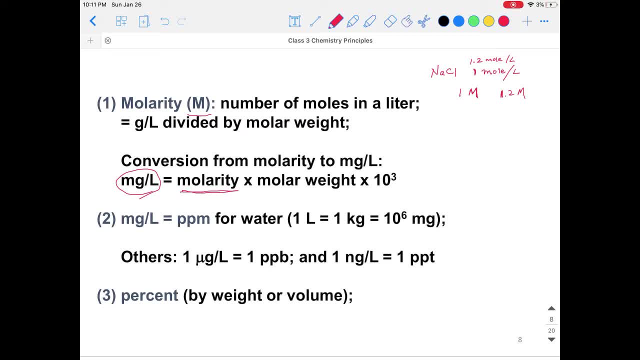 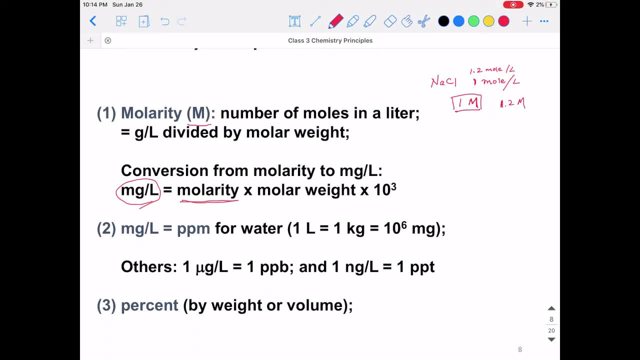 milligram per liter. So in this case we know that for sodium chloride, let's say that the molarity is one M, then we know that sodium chloride has a molecular weight of 23 plus 35.5, which is equal to 58.5 gram per mole. So how do we calculate the 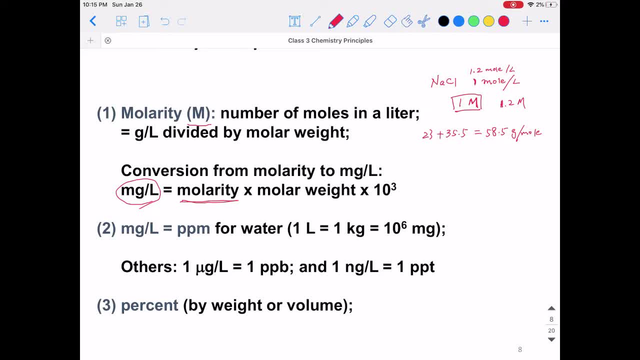 um. mass concentration of sodium chloride in the liquid. So that can be quite easily calculated by um. so basically, the mass concentration, let's say this is defined as x, we want to represent its in the unit of milligram per liter. So that's going to be one M. So we know that one M. 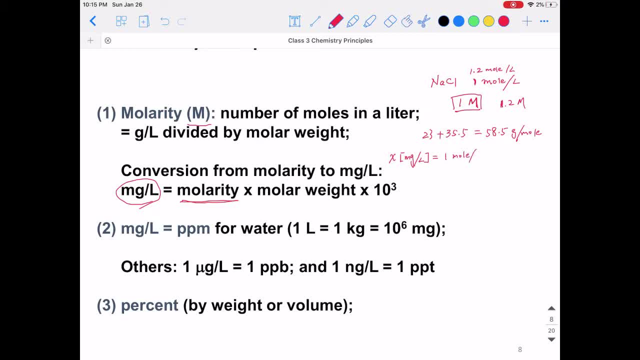 is equal to one mole per liter, right? And then we're going to multiply the uh, the molecular weight of sodium chloride. that is 58.5 gram per mole. So we can see that in terms of the unit mole can cancel out, which is going to be equal to 58.5 gram per liter. So please notice that here. 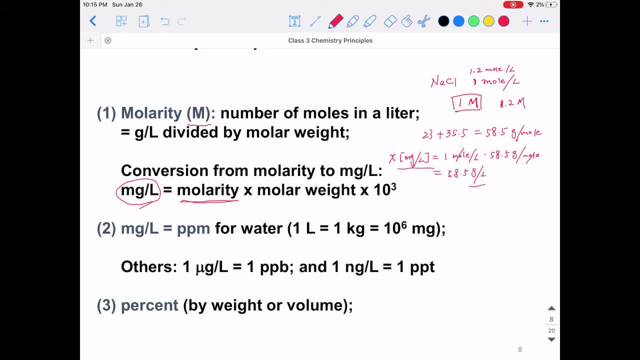 the units are a little bit different, right? So we want to convert it into milligram. milligram per liter, So we're going to multiply by 1000, right, So that's going to give us um, um, um. 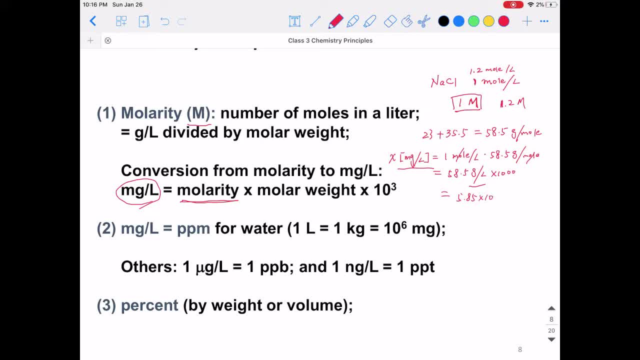 5.85 multiplied by 10 to the fourth milligram per liter. So this is how we can um, based on this equation, to calculate or to convert the um molarity into uh mass concentration And in terms of the mass concentration shown in milligram per liter. 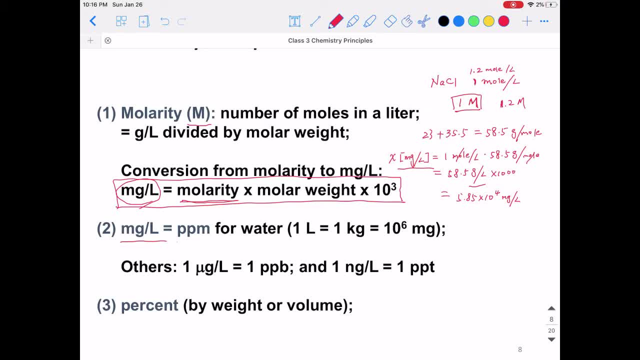 we can also notice that, or we can, or we can also also call that as ppm for water. So, for example, um, if we prepare a solution that's containing one m of the sodium chloride, then we can know that. we can also say that in this. 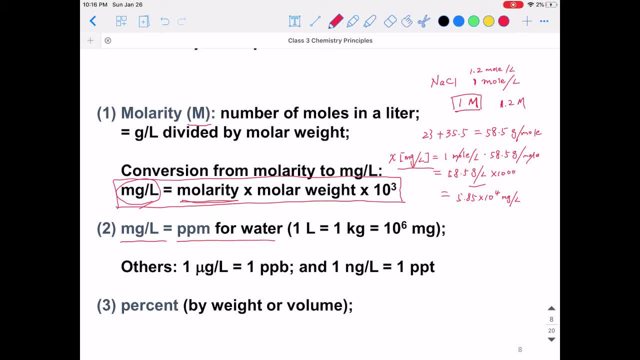 sodium water uh solution, we're containing 5.85 point 10, um multiplied by 10 to the fourth ppm of sodium chloride. So why is it? That is because, if we try to represent the uh uh, 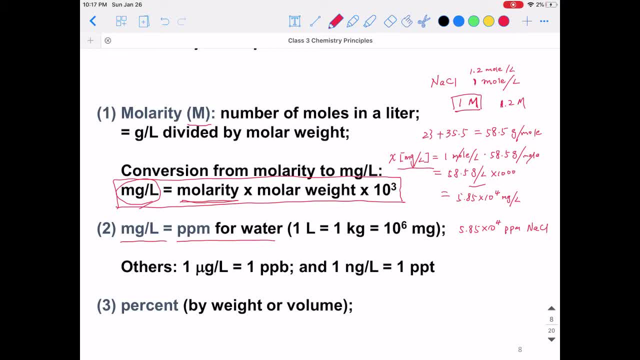 mass fraction. So basically we're converting this mass concentration into the mass fraction shown in ppm. So we first need to convert the liter here into the mass of water, right? So for dilute solutions one liter represents 1000 grams, right? We also know that one milligram 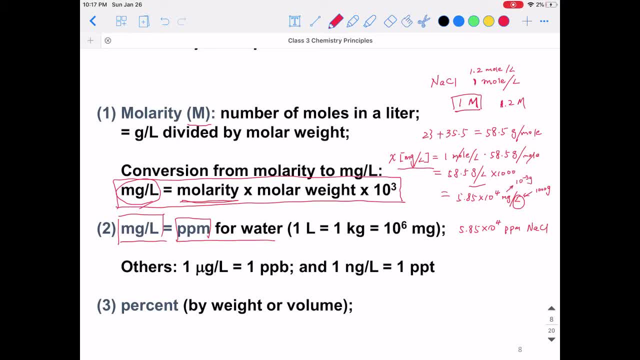 represents 10 to the minus 3 grams. So basically, one milligram per liter is equal to 10 to the negative 6 grams of the solute over grams of the water. So what this means is that one milligram per liter is approximated by one ppm of the solute. 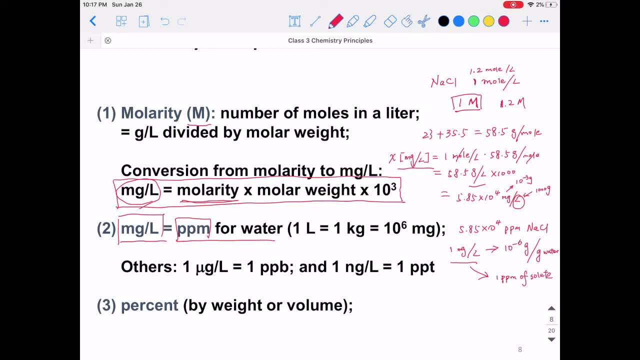 So this is how we can convert the mass concentration into the mass fraction of the solute right And, for example, for the other units, for example, we're having a further lower value, or further lower, smaller value of the mass concentration, Then one microgram per liter is. 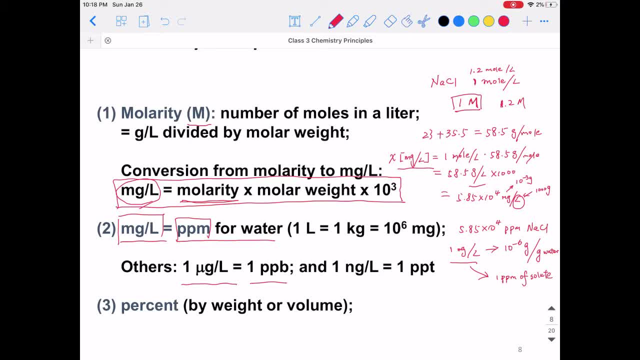 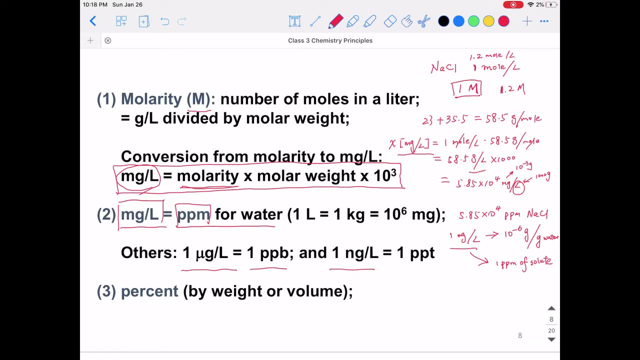 equal to one ppb, because ppb is parts per billion, right? So that's 10 to the negative 3 of the ppm, And one nanogram per liter is going to one ppt, Which means one parts per trillion, So to represent the concentration of the solute in water or other species in water. 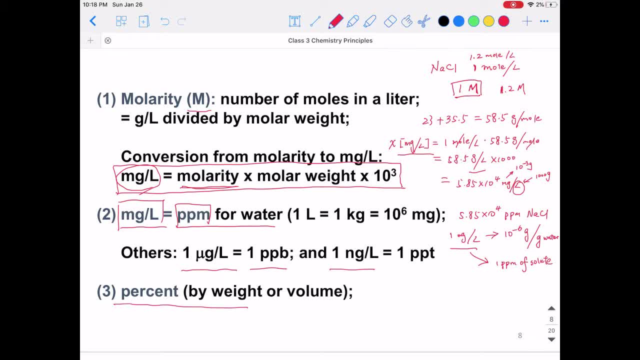 we can also use the percent, and that can be either by weight or by volume. So if it's by weight, then we're talking about the fraction again. So you know that for one ppm in terms of weight, then that means 10 to the negative, 6 in terms of the mass fraction, right? 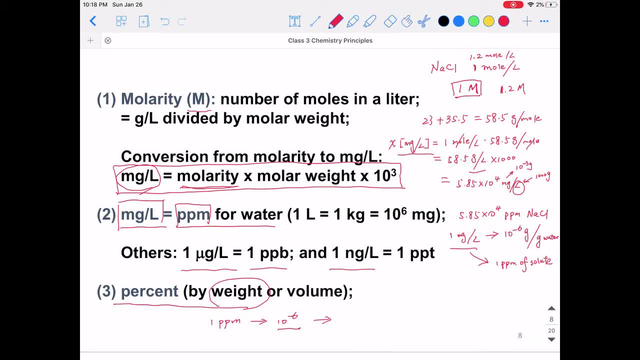 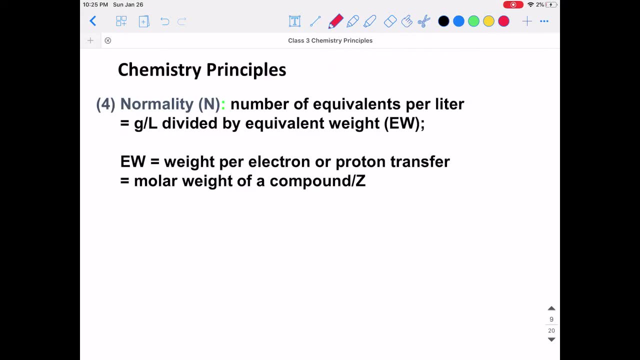 If we further try to represent that into percent, then that's going to be 10 to the negative 4 percent. right, Because one percent is 10 to the negative 2 in terms of the fraction. So now we can get into the definition of normality, And I have to mention that normality is: 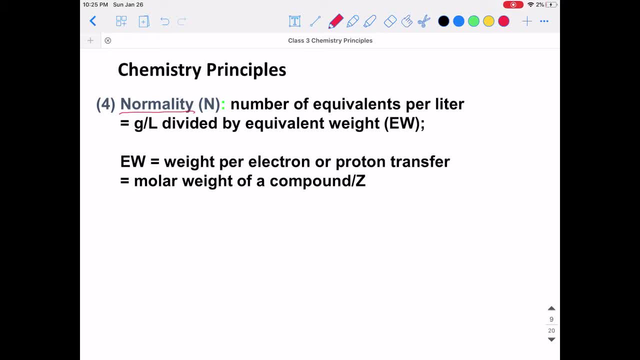 a quite complex definition but if you follow me step by step you will see that how we can use that In environmental engineering right. So by definition the normality means the number of equivalents per liter. So this equivalent can be anything right It can be using. 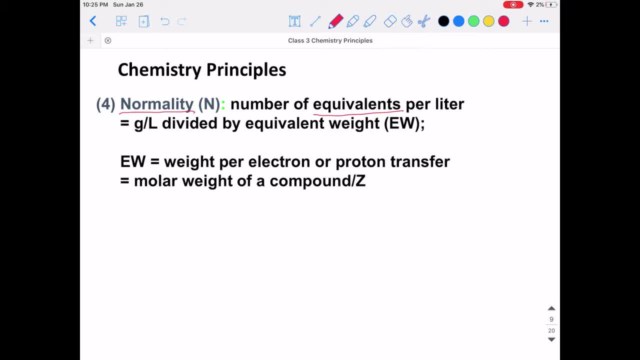 any references. For example, it can be hydrogen, right In water treatment. we want to use calcium carbonate, right. It also can be sodium chloride or it can be anything. So it means the number of equivalents per liter and that can be the number of equivalents per liter And that can. 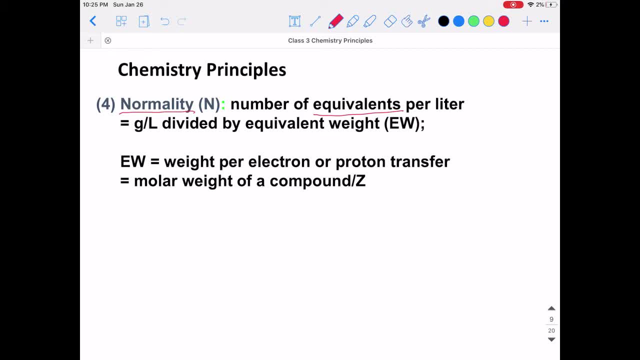 be in reference to any chemicals, And the normality is also calculated by the mass concentration of the species. For example, we're talking about the sodium chloride again, and they're divided by the equivalent weight. Okay, and then the equivalent weight, as you can. 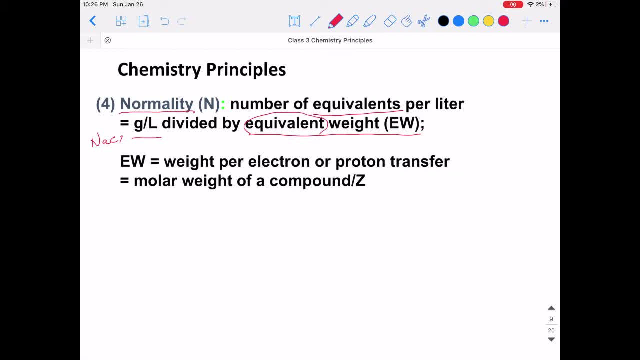 see that should be in terms of other species. So the equivalent weight is calculated by the weight per electron or primary. So I'm still asking myself some questions If, oh, that means the number of equivalents per liter is the same as what we have for juice ح? Yes, let me just add. 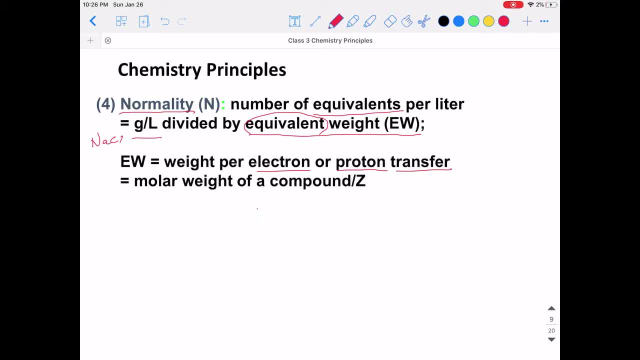 expand that so that I can see. So fuel completeness is more or minus theна proton transfer. For example, if we're talking about NaCl again, then this number, this electron or proton transfer, is going to be equal to 1.. And then, if we're talking about 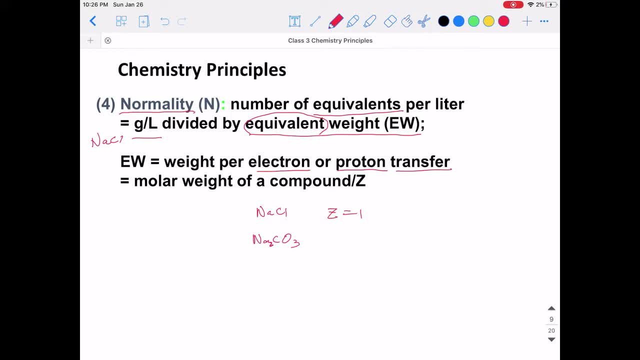 sodium carbonate. we know that there are two electrons basically carried by the carbonate ion. then z is going to be equal to 2. And we can also apply this into the oxidation reduction reactions and that also concerns the electron or proton transfer from these. 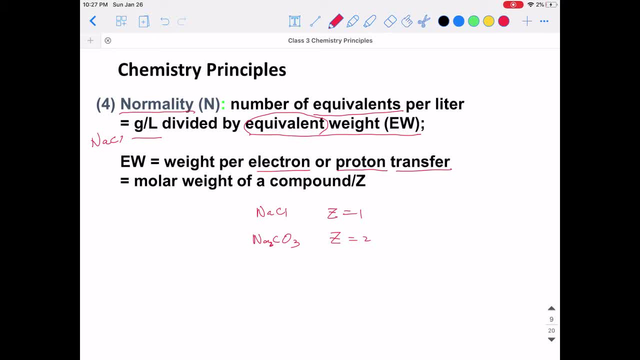 oxidations or from these chemicals. So the equivalent weight is calculated by dividing the molecular weight of a compound. so that can be of any compound. Let's say we mentioned about the calcium carbonate, we mentioned about the hydrogen there. so that is calculated by dividing the molecular weight of that compound by the number of 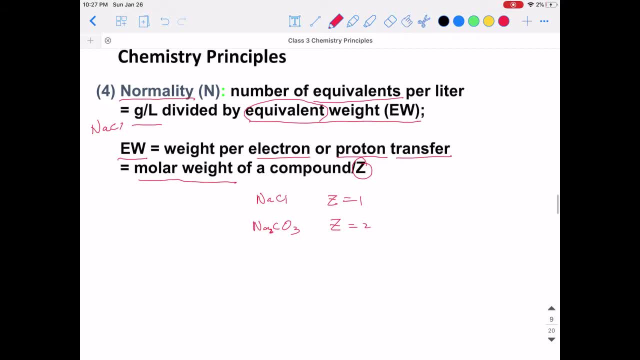 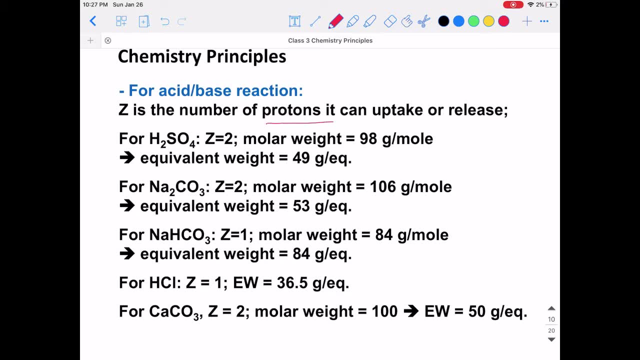 electrons or proton transfer. So here I can give you some more examples. For example, for the acid-base reaction, the z is the number of protons it can uptake or release, For example if we're talking about the sulfuric acid. so we know that the sulfate ion carries two charges. 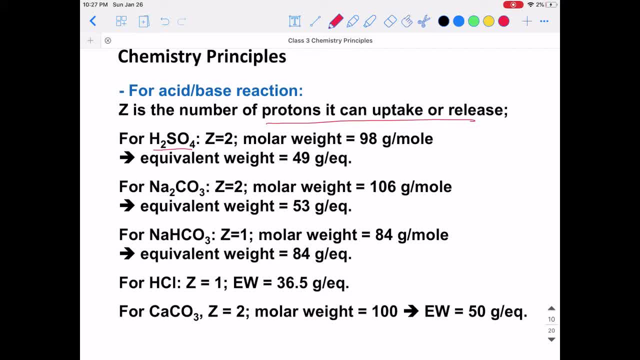 that is going to probity. the second union, the z should also, like I said, is taken. So, under this situation, the z, which is a number of protons or electrons they can provide or release, The z is going to be equal to 2.. 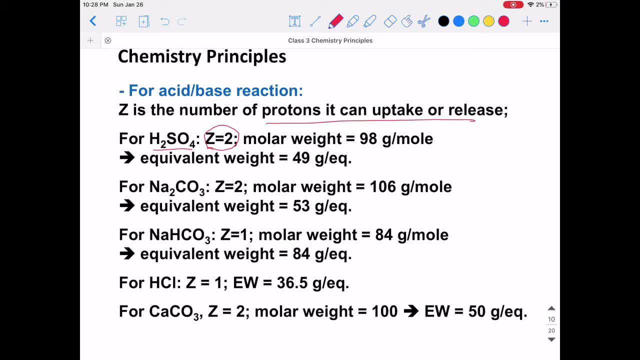 and then we know that the molecular weight of the sulfuric acid- let's do a quick calculation- that's going to be 1 multiplied by 2, plus 32, plus 16, multiplied by 4.. So that's equal to 34. 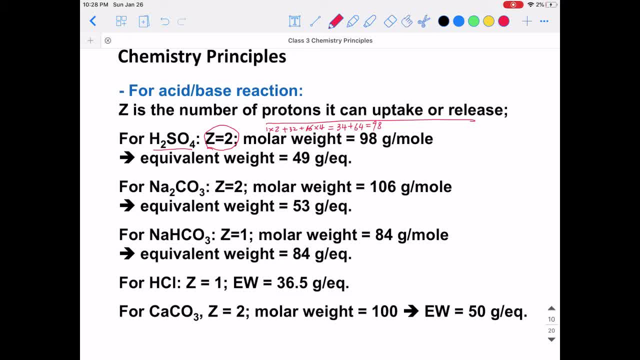 64 plus 64,, which is giving you 98 gram per mole, right? So under this situation, the equivalent weight for the sulfuric acid is going to be 98 divided by 2, which is 49,, right? So this is if we want to represent its unit. that's also shown as gram per equivalent and we're showing this abbreviation here. 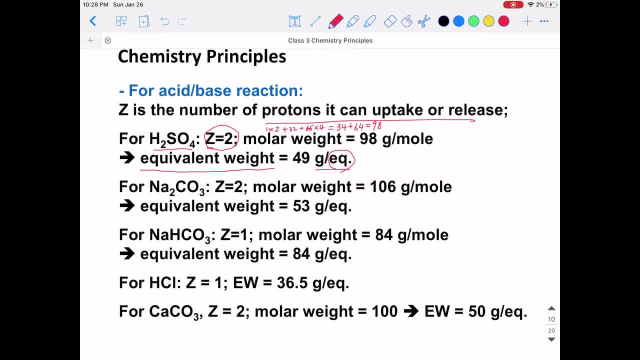 And for the sodium carbonate, similar to the sulfuric acid, Z is equal to 2, because this is mainly contributing from the carbonate ion. So under this situation, the molecular weight for the sodium carbonate- so let's do another calculation, right. 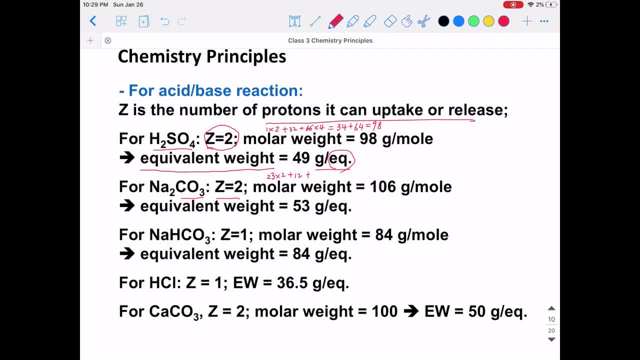 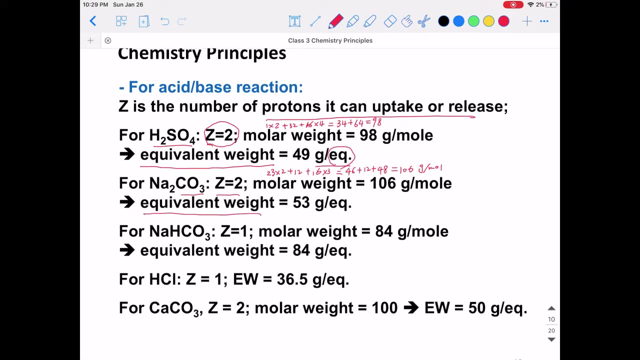 So 23 multiplied by 2 plus 12, plus 16 multiplied by 3.. So you have 46 plus 12 plus 48.. So this is going to give us 106 gram per mole, And so since the Z is equal to 2, then the equivalent weight for the sodium carbonate is going to be 53,, which is 106 divided by 2.. 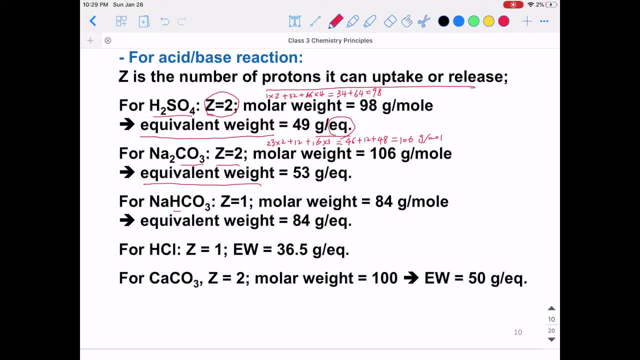 And for the sodium bicarbonate we see that sodium carries one charge right And bicarbonate ion carries one negative charge. So Z is equal to 1. And the molecular weight is 84 gram per mole. So the equivalent weight for the sodium bicarbonate is 84.. 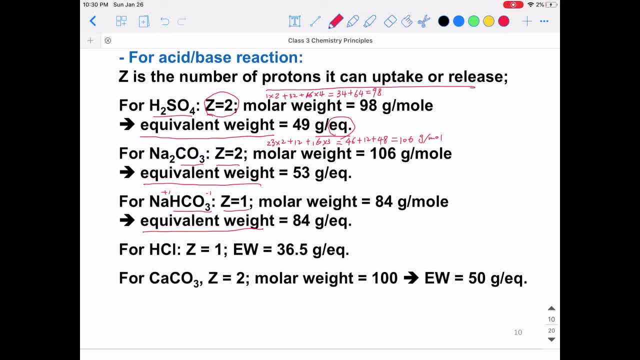 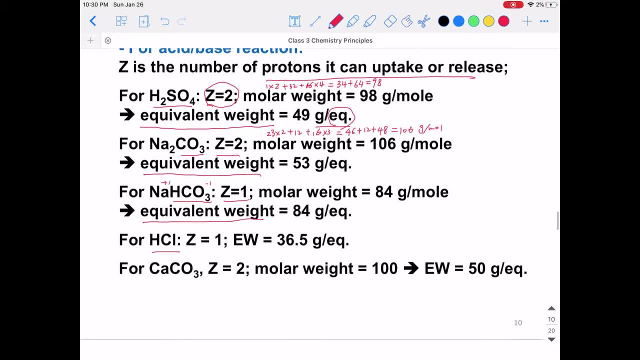 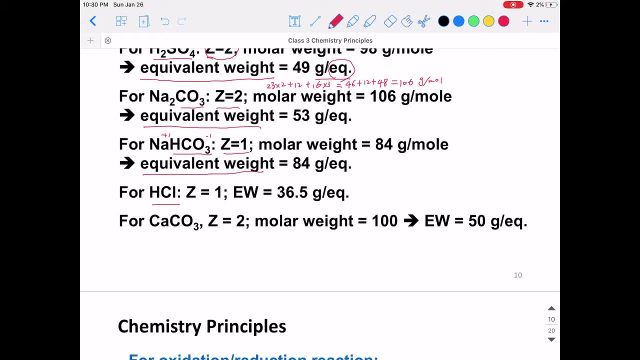 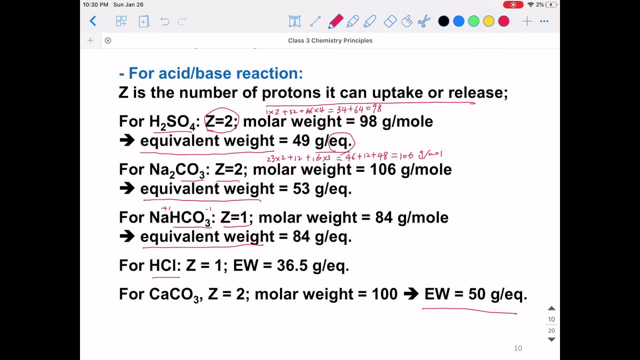 And for the hydrogen chloride right. So we have the Z equal to 1, and then the equivalent weight equal to 36.5.. And the calcium carbonate is going to give us an equivalent of 50 per equivalent right. So with the definition of the equivalent weight, then we can calculate what normality really means. 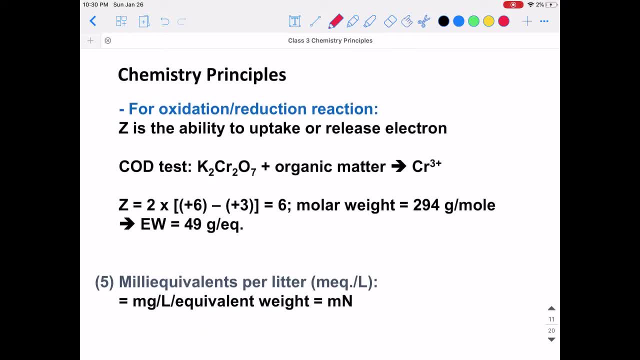 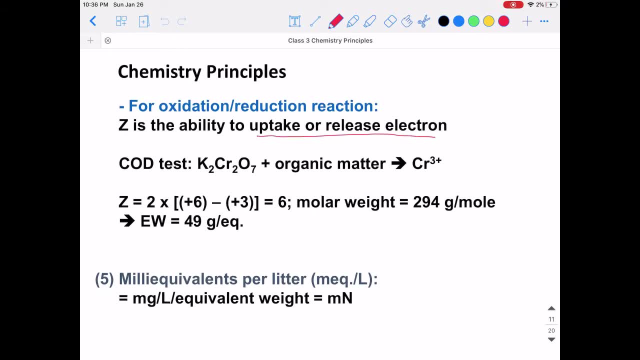 And similarly for the oxidation reaction, oxidation reduction reactions. Z is the ability to uptake or release electrons. So typically we're going to use the potassium dichromate for the COD test. So COD here represents the chemical oxygen demand. This is a parameter that basically relates to the quality of the water. 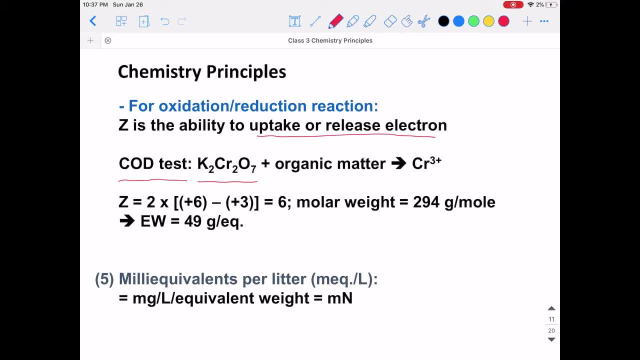 So we're going to use this chemical to oxidize certain organic matter in the water. So after the oxidation, the chromium is going to be reduced into the oxidation state of plus 3, right? So let's see what is the number of electrons being exchanged within this chemical. 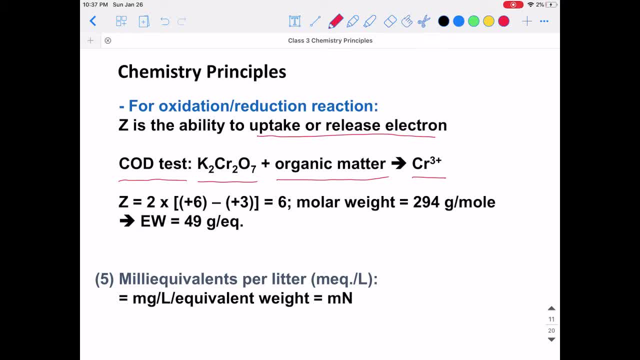 So before the oxidation reduction reaction. so we know that potassium is providing plus 2 of the oxidation states, right. And then the oxygen is providing negative 14, because we know that all the oxygen is going to be in a state of negative 2, right. 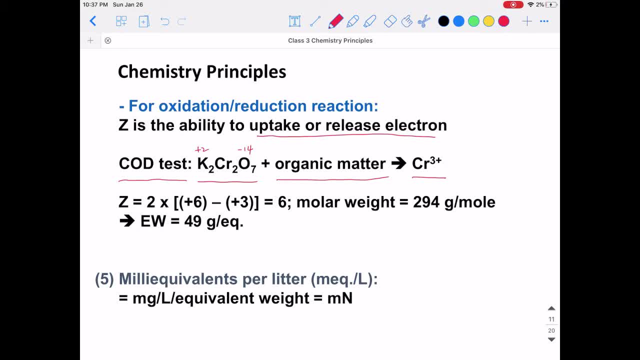 So the two chromium elements or atoms here are going to cover an oxidation state of plus 12.. So each of them is going to be an oxidation state of plus 6, right? So after this oxidation reduction reaction, the chromium is going to be reduced to plus 3.. 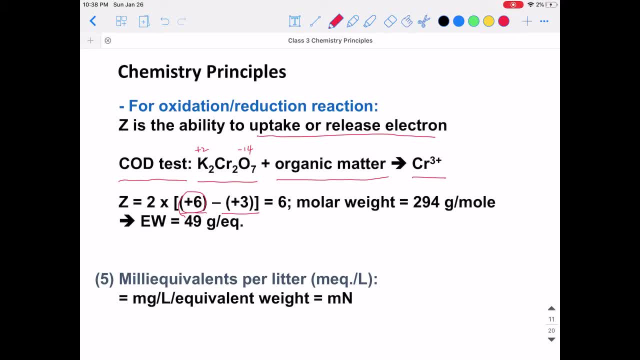 So what that means is that there is a net exchange of electron, or three electrons per chromium atom. So there are two of them, which means that the Z here is going to be 2 times 6 minus 3, which is going to give us a number of electrons of 6.. 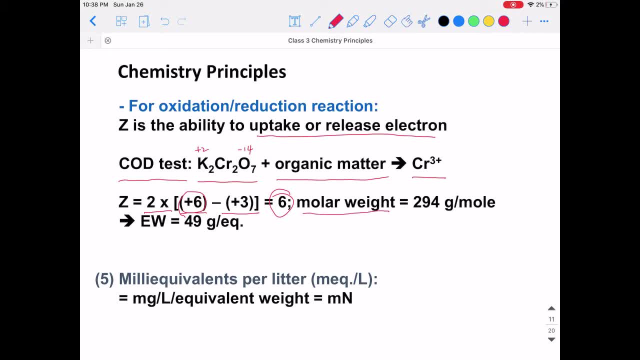 We also know that the molecular weight of the potassium bichromate is equal to 294.. So this is going to do This is going to give us an equivalent weight of 294 divided by 6, which is 49, okay. 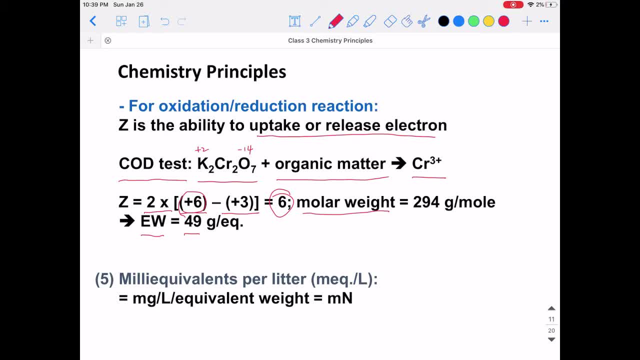 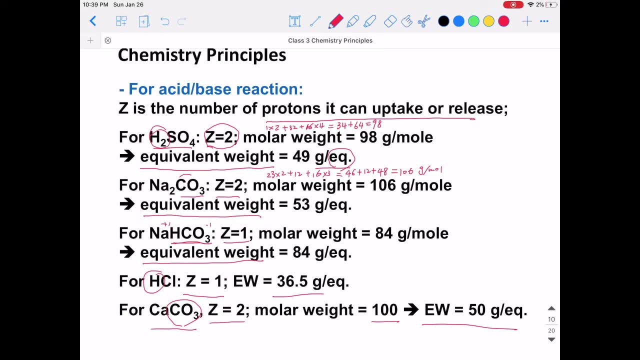 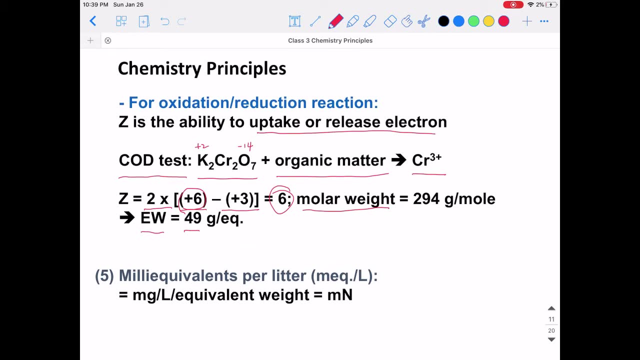 So this is how we can calculate what is the equivalent weight for a single species for the oxidation reduction reaction. So you can see the difference from the calculation for the acid-base reactions, And we can also use the parameter of the milliequivalence per liter. 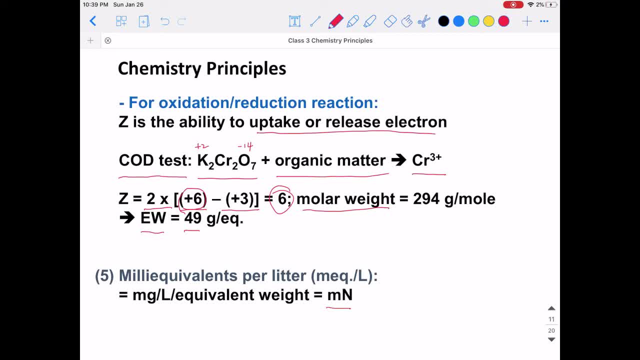 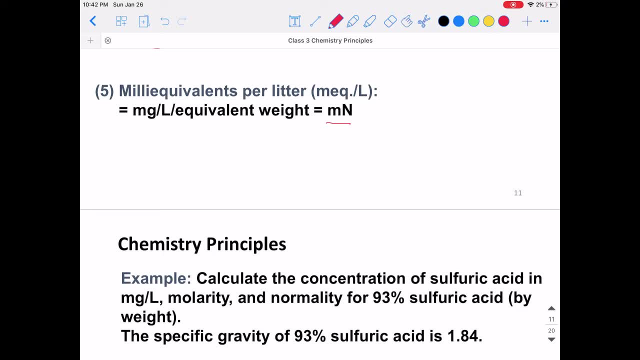 So basically, milliequivalence per liter means 10 to the negative 3 of the molarity. So how do we apply these different units into the analysis of a solution? So here I give an example. So it wants us to calculate the concentration of sulfuric acid in milligram per liter. 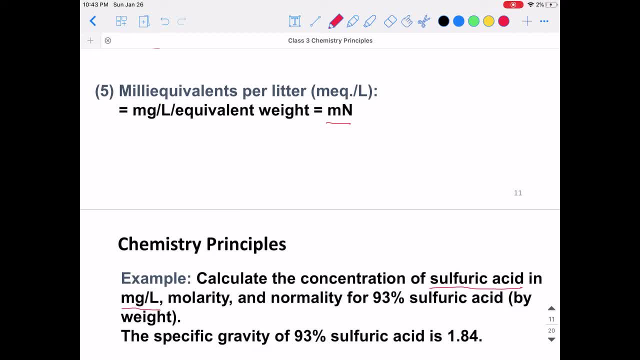 So also notice that for diluted species or diluted solutions milligram per liter also is equal to ppm, right Also in molarity and normality for 93% sulfuric acid. So the remaining sulfuric acid. So the remaining sulfuric acid. 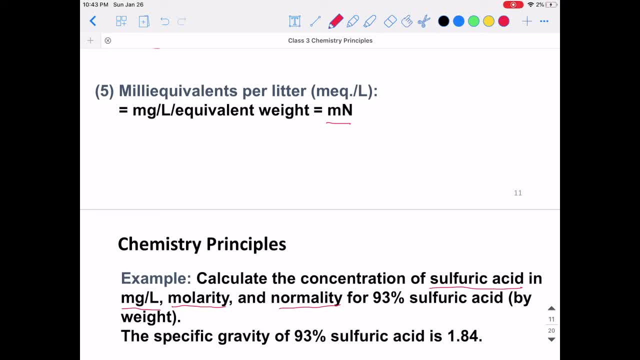 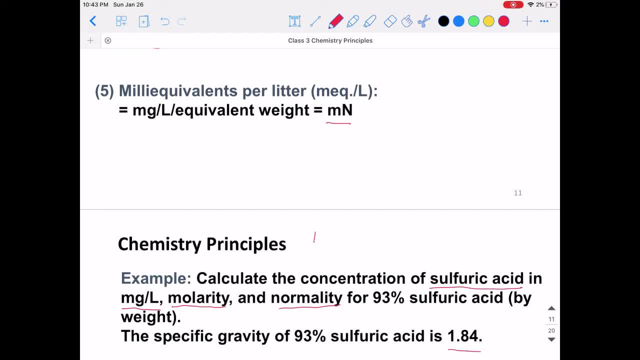 So on the 확인Ing side you can see that this solution contains a density of 7% of water, So it has a specific gravity of 1.84.. So what this means is that the density of this solution is 1840 gram per liter. right. 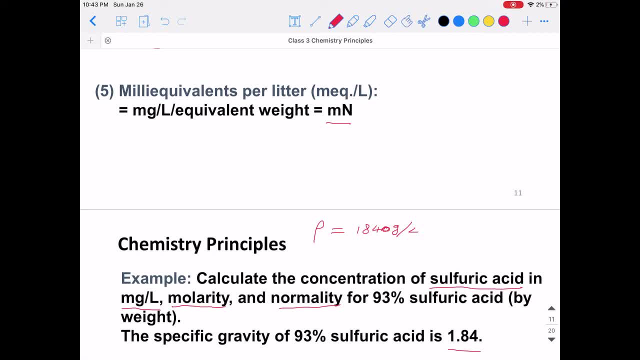 So because we know that the specific gravity is in terms of the water, right. So water has a density of 1 kilogram per liter, which means that the density of the sulfuric acid solution is going to have this value here. so further, we know that 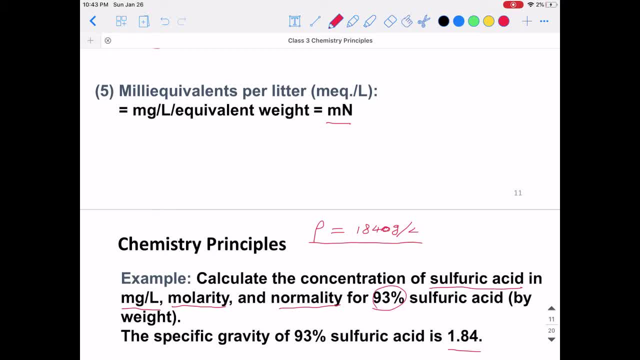 this solution contains 93% of the sulfuric acid. so now we know that if we want to show the mass concentration, then we have to calculate based on the density, because 93% of them is going to be represented by the sulfuric acid, and further we can convert. 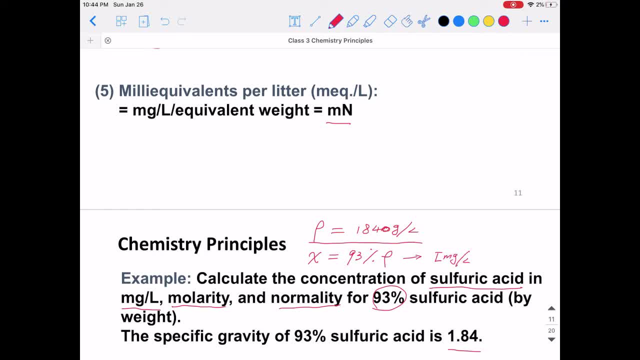 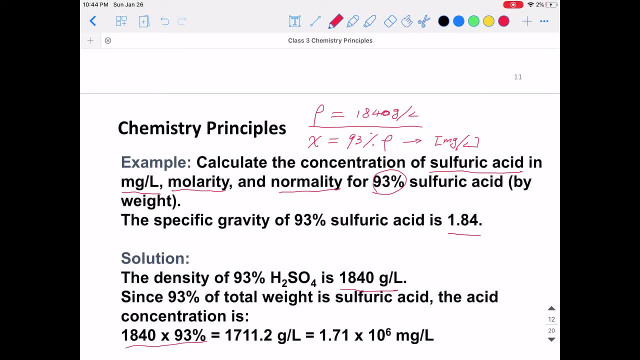 this unit into the values in milligram per liter. so this is how we can solve it. so we have 1.840 and then we multiply that by 93% and this is going to give us 1711.2 gram per liter further. we want to show these. 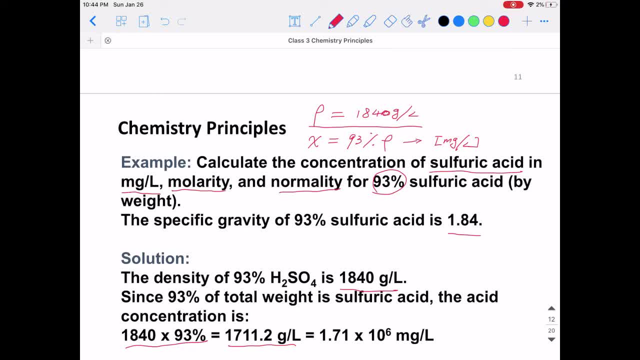 values in milligram per liter. so that's why we have to further multiply these values. so that's why we have to further multiply these values, so that's why we have to further multiply by 10 to the third to show the values in milligram per liter. so then, since 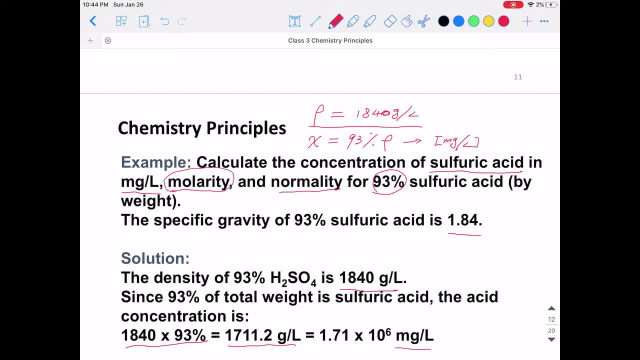 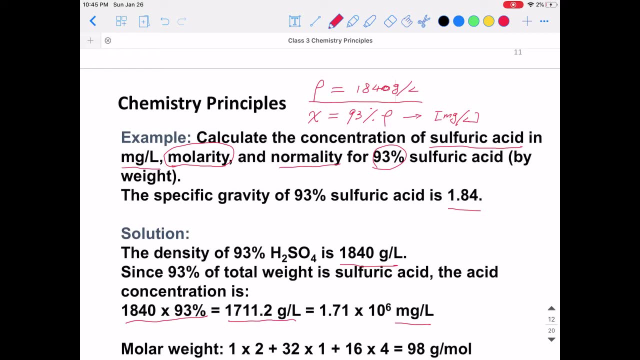 we have the mass concentration. how do we calculate molarity? so we can directly use the mass concentration and divide that by the molecular weight of sulfuric acid to get molarity. so basically we have to calculate what is the molecular weight, as we have shown before, the molecular weight of sulfuric 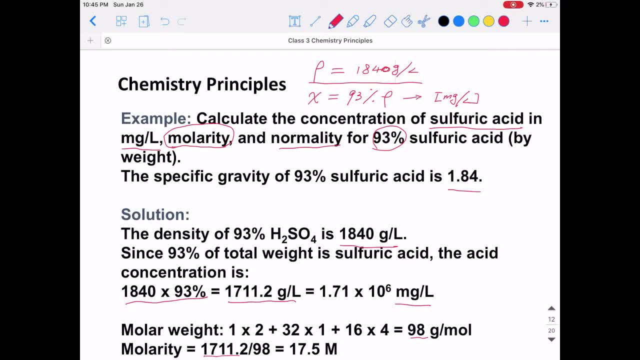 acid is 98.. in order to calculate molarity, we can directly divide that. divide the mass concentration by 98, and that is going to give us 17.5 m, which is showing in the molarity and in terms of the normality. we know that this is basically for the 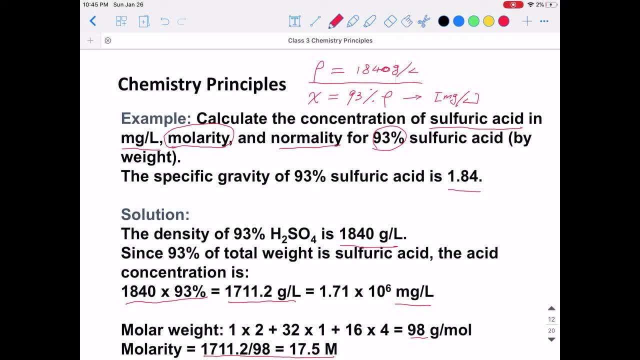 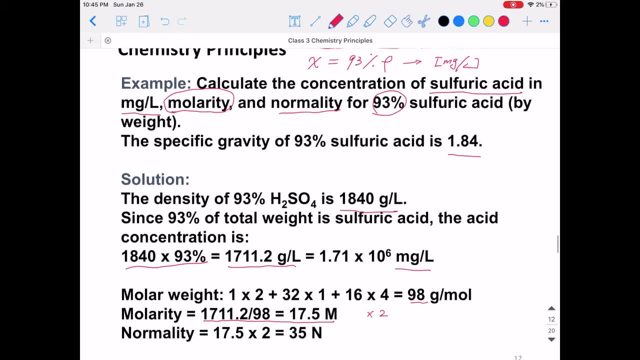 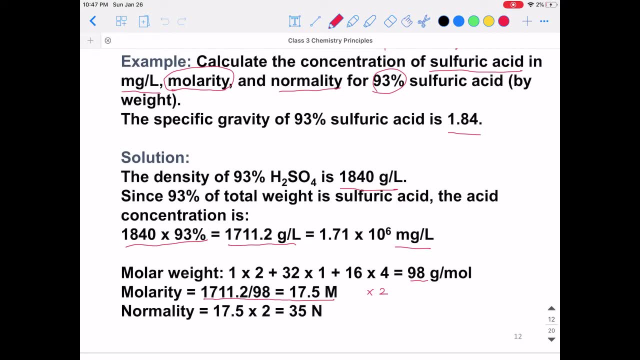 sulfuric acid. it's providing two protons, right. so considering that it's providing two protons, then we just need to multiply that by 2.. and then that is giving us a normality of 35.. so now let's go back to the definition of. 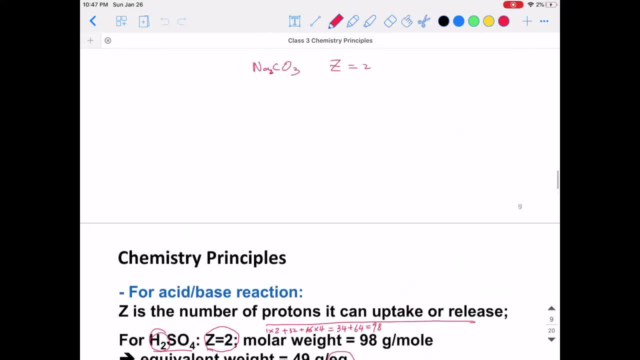 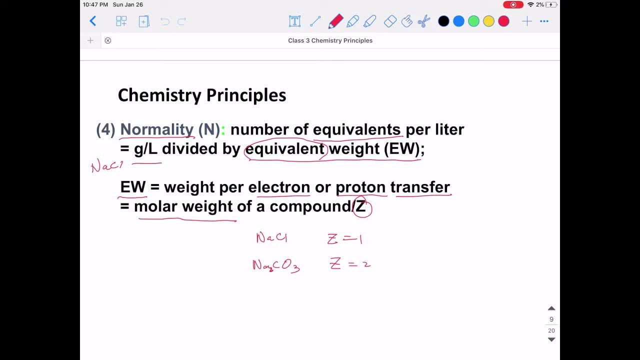 the normality and see what that really means. so, in terms of the normality, it is defined as the number of equivalents per liter, right, so it can be calculated based on mass concentration divided by the equivalent weight. as we have shown, the equivalent weight can have different values, right, depending on how. 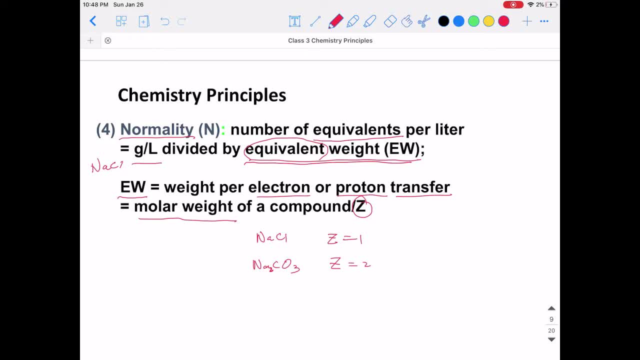 many protons are being accepted or released for the acid-base reactions, or how many electrons are being released or accepted in the oxidation-reduction reactions. and because for the sulfuric acid the equivalent weight is half of the molecular mass, which is 48, then that's why we can basically multiply the molarity just directly by 2, to get the 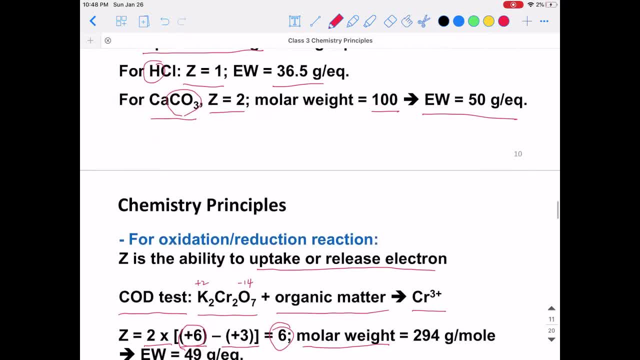 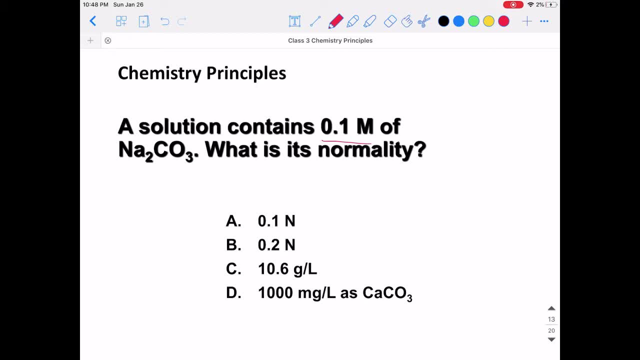 normality here. so now let's do a quick quiz here. so if we have a solution that contains 0.1m, so notice, this is the molarity of the sodium carbonate. so what is its normality? the normality is going to be equal to 0.2n here. 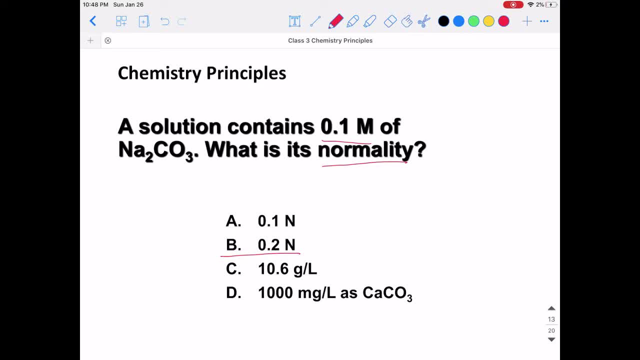 so basically we can do that in a complex way because we know that the molecule weight of the Sodium chloride is going to be 46 plus 12 plus 48, which is 106 gram per mole. So we can first convert this molarity into mass concentration, and that can be quite. 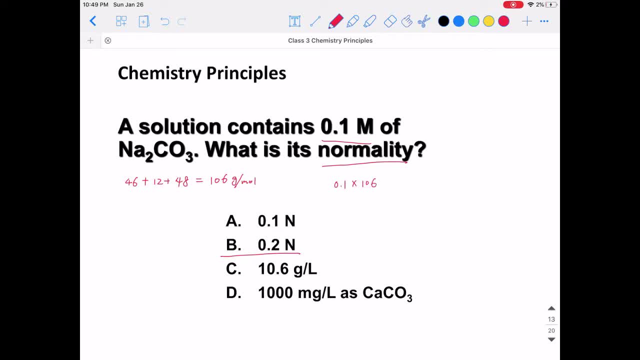 easily done by just using 0.1 multiplied by 106.. So this is giving us 10.6 gram per liter. So what is the equivalent weight of sodium carbonate? That is 53,. right, Because it's going to be able to accept two protons. 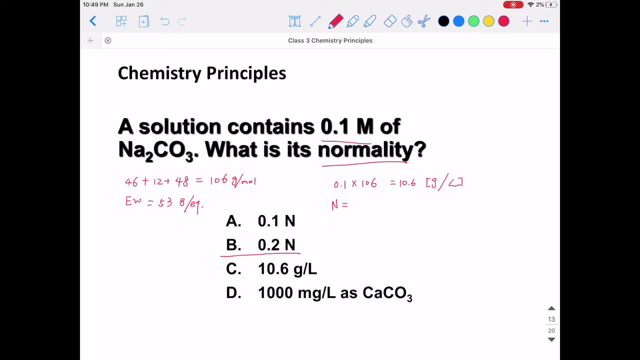 So the way we calculate normality, n is going to be equal to the mass concentration, 10.6, divided by 53, which is basically equal to 0.2n here. okay, Or we can just think of that in a more simpler way, because since we already know that the 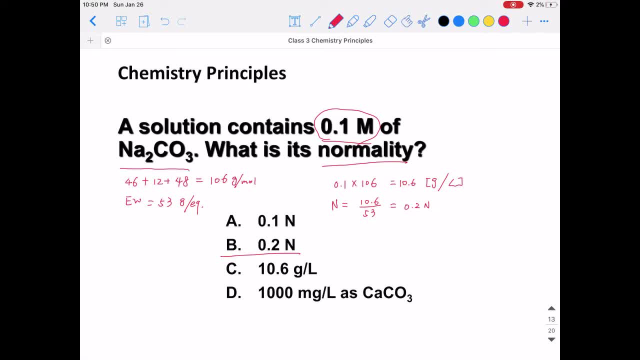 molarity is 0.1, and we know that there are two charges or two protons that can be accepted, then its normality is just going to be two times or twice of the molarity Which is 0.2n. 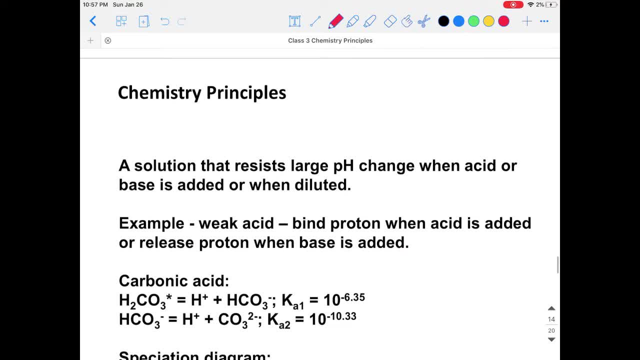 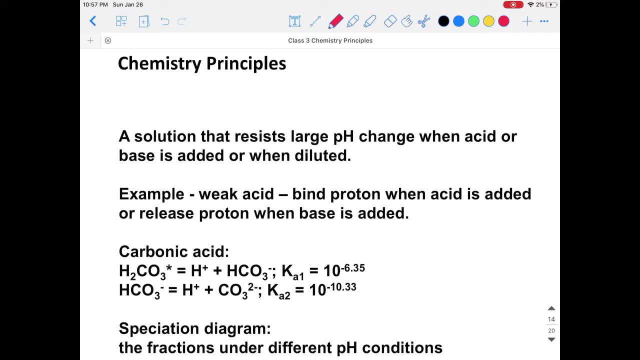 And now we can take a look at the buffer system. So what is a buffer? A buffer is a solution that can resist large pH changes when the acid or base is being added or when it's being diluted, And, for example, a weak acid can be a buffer, okay, 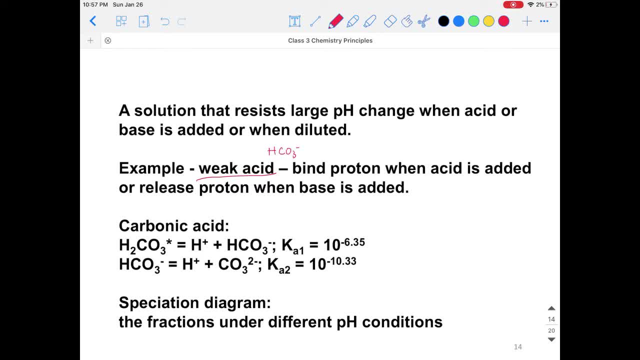 So let's take the bicarbonate ion, for example. So basically for bicarbonate ions. So basically for bicarbonate ions. So basically for bicarbonate ions, Or for a solution that's containing bicarbonate ions if we add hydrogen chloride into the. 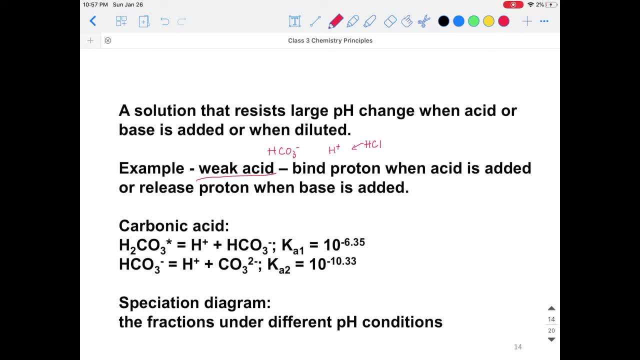 solution, then the protons being released from the hydrogen chloride can bind with the bicarbonate ion and we're going to form the carbonic acid. okay. And if we're adding some base into the system, for example sodium hydrochloride? 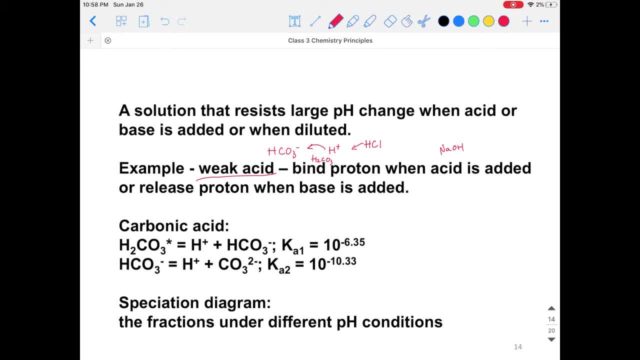 Okay, Right, So then these OH radicals or OH ions can react with the bicarbonate ions And then we're basically going to form water and carbonate ions, right? So in this way the pH can be buffered, So the pH is not going to directly get reflected from what is the concentration of the protons or the OH ions here. 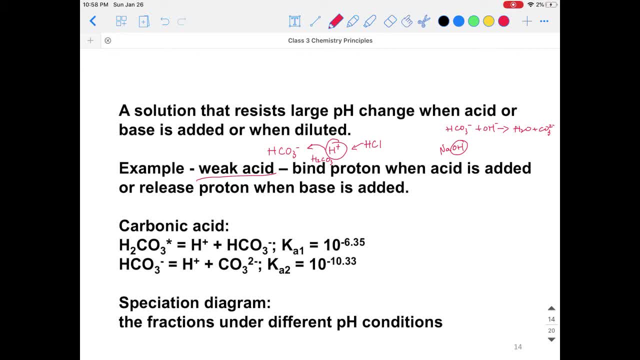 Okay, So that is why the carbon dioxide, or the carbon dioxide bicarbonate ion or carbon ion, can form a buffer solution, And this is related with a series of reactions. So, for example, the dissociation of the carbonic acid. right, So we know that the dissociation of the acid can give us one proton and one bicarbonate ion. 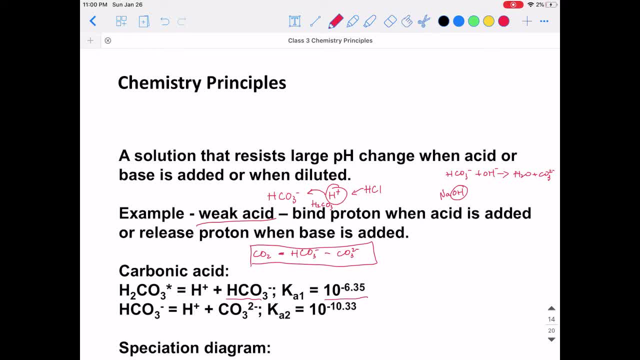 And this reaction has an equilibrium constant of 10 to the negative 6.35.. And in terms of further dissociation of the bicarbonate ion, it can get dissociated into a proton again and a carbon And for this reaction it has an equilibrium constant of 10 to the negative 10.33.. 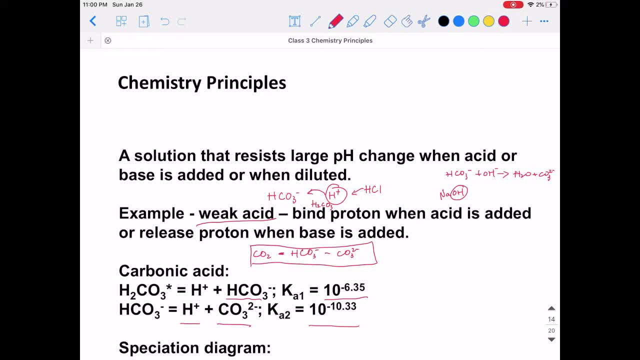 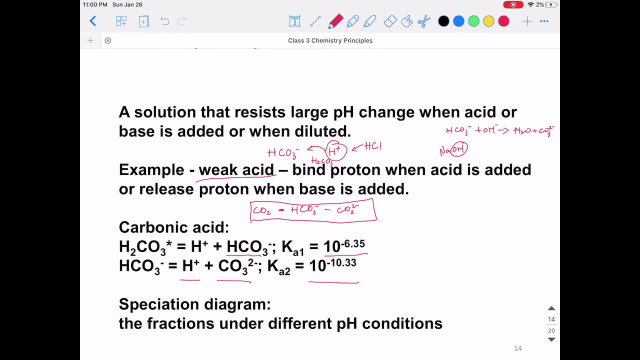 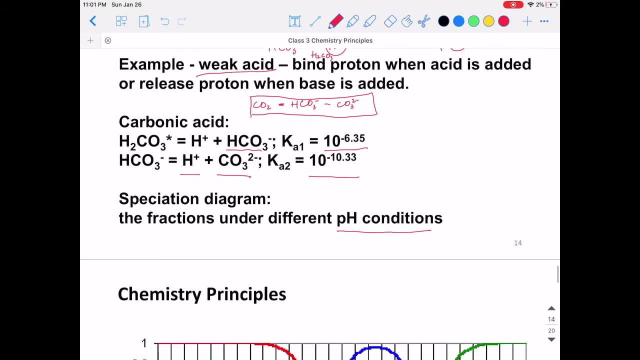 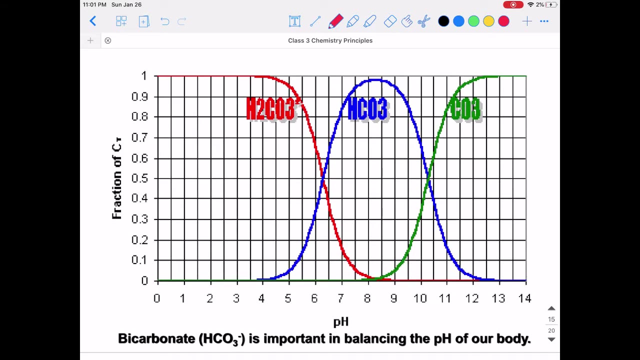 So how does this affect the pH or affect the buffer system? Okay, So from this series of dissociation reactions we're going to basically generate ions. that's dependent on the pH conditions, And here is showing a basic diagram That's representing or showing the concentrations of these three different species under different pH values. 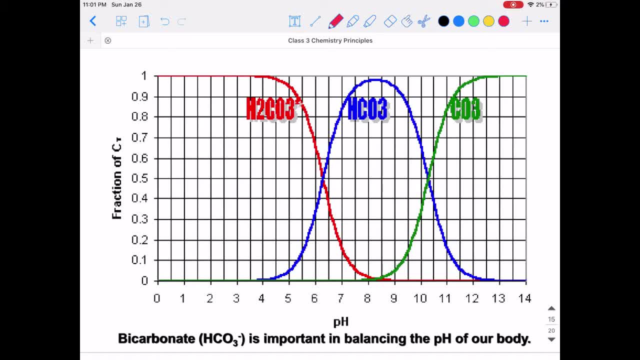 So you can see that under very high acidic conditions or low pH value conditions, then the solution is going to be mainly composed of the carbonic acid right. So as the pH further increases, we're going to see the formation of the bicarbonate ion right. 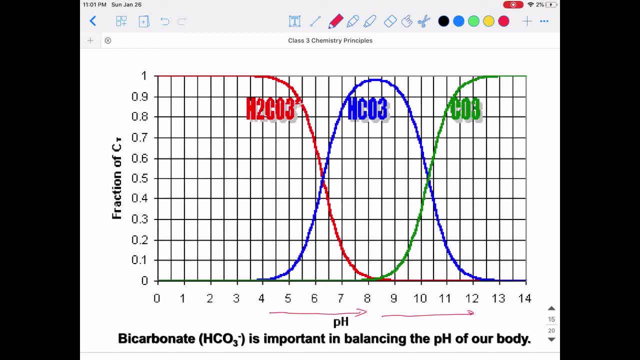 And as we further reduce the pH, we're going to see the formation of the bicarbonate ion, the pH, for example, by adding OH ions into the solution, and then the bicarbonate ions are going to get reacted and finally form these carbonic carbonate ions. okay, and we have to mention that bicarbonate 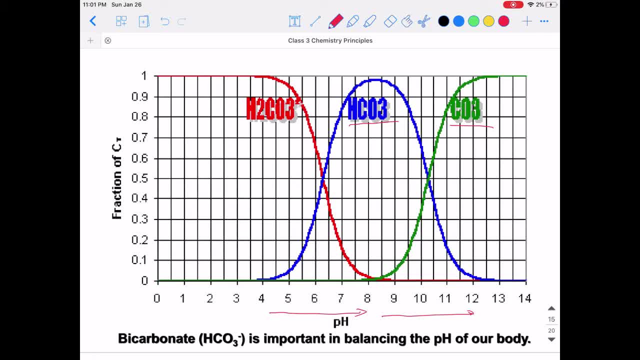 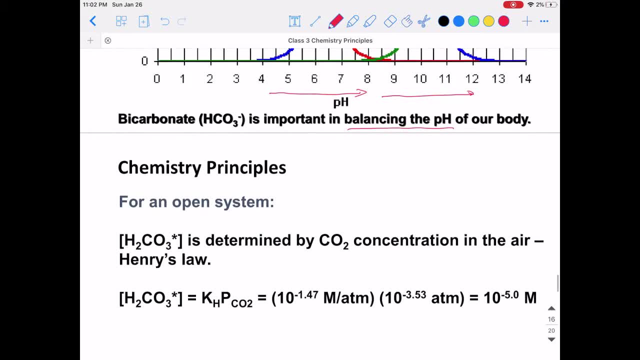 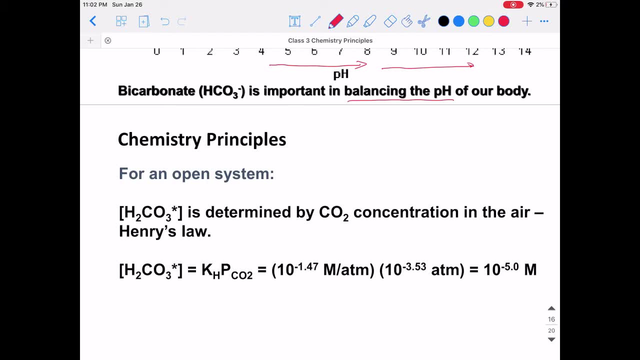 is very important. so this buffer solution is very important in our body, that is, balancing the pH. okay, so without this system, our body cannot function well. so, with this information, how do we solve or how do we look at the typical mixtures in the nature? okay, so for an open system, as we have. 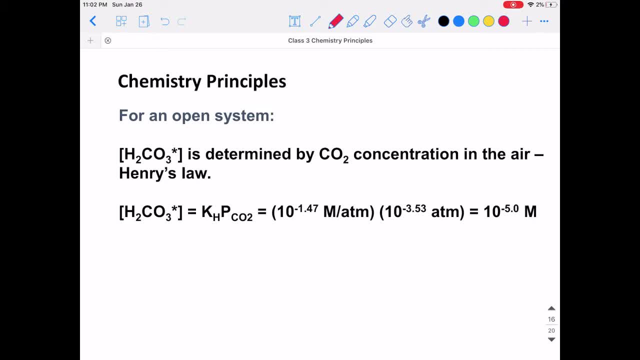 learned from our previous lecture. we know that the concentration of the carbonic acid is purely dependent on the carbon dioxide concentration in the atmosphere, and this is decided by the Henry's law right. so we know that we can find out that Henry's constant for the carbon dioxide. 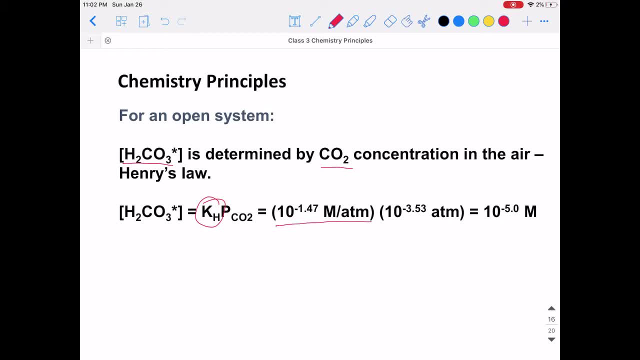 So this is providing us a value of 10 to the negative 1.47 m per atmosphere, And we also know what is the partial pressure of the carbon dioxide in the atmosphere. So basically, based on the Henry's law, we can calculate what is the concentration. 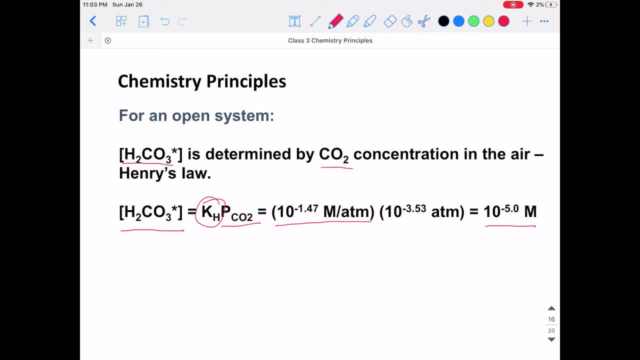 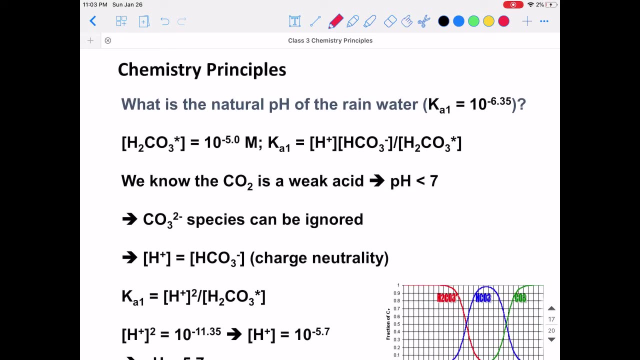 of the carbonic acid in water. So that's going to give us a concentration of 10 to the negative 5 m, And so again, m is equal to mole per liter. So how can we apply this into the calculation for the pH of rainwater? 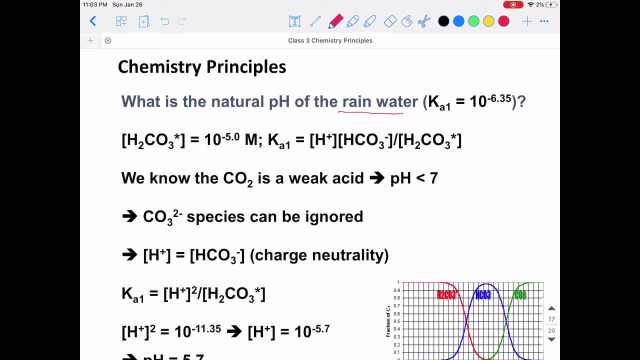 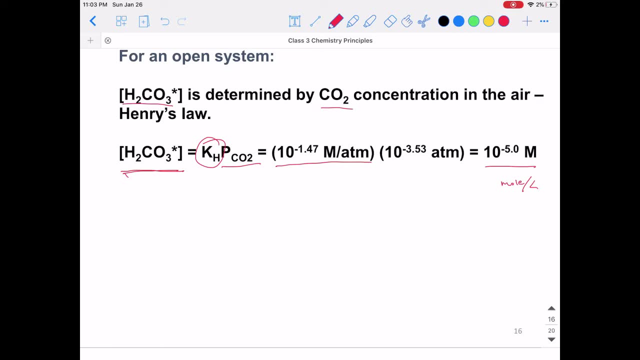 So, if you consider for the rainwater, there is a complete contact between the liquid and the gas environment And since our atmosphere contains carbon dioxide, which is the reason why we're having a certain amount of the carbonic acid in the solution, 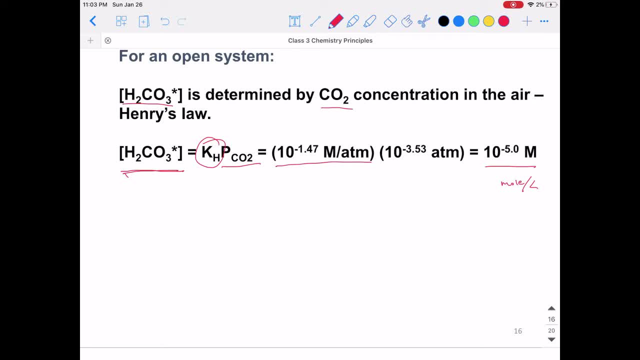 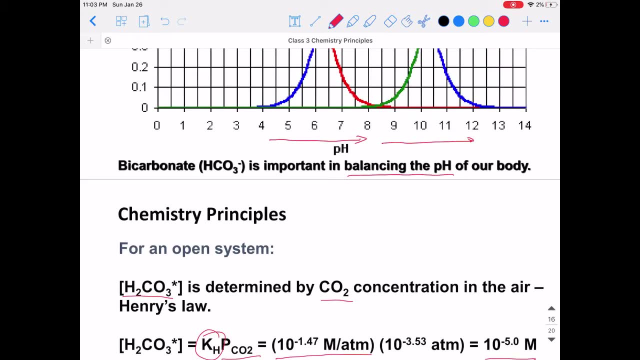 so this is going to give us a lower pH. So what this lower pH means is that the pH of this solution, or pH of this rainwater, is going to be lower than 7, because we know that 7 is neutral condition. 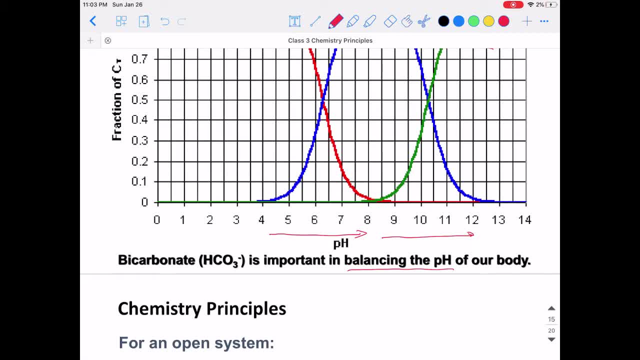 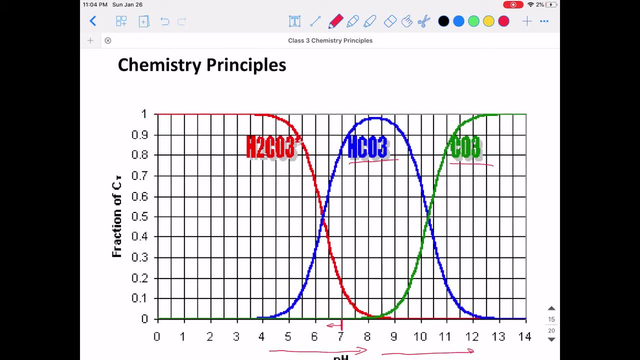 It doesn't have any other ions, just purely hydrogen and the hydroxide ions. OK, So by having this condition, we know that if the pH is below 7, then there's no carbonate ions, So the solution is mainly just composed. 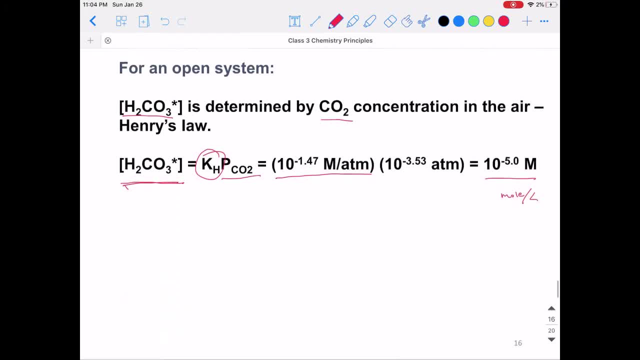 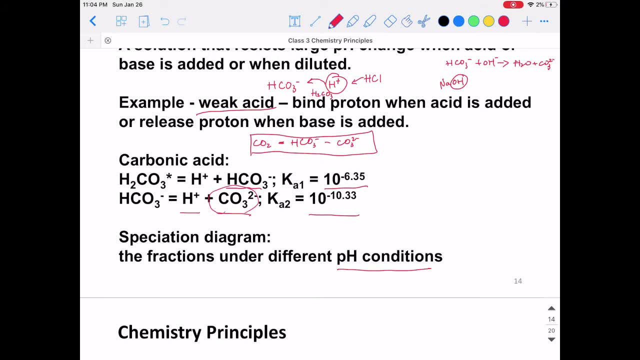 of the carbonic acid and the bicarbonate ion. So now we can use the relationship of the dissociation reaction for the first reaction here, because we can basically ignore this reaction since pH is lower than 7.. So this is how we can solve it. 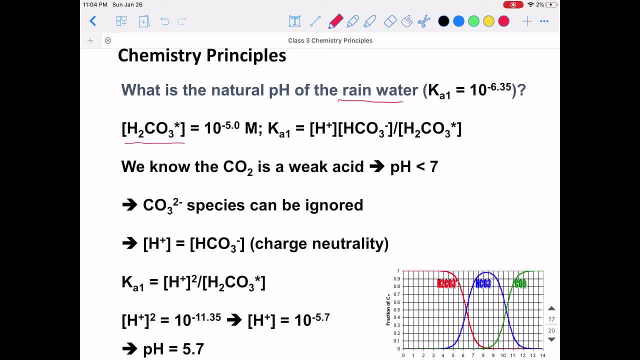 So, since we already have the concentration of the carbonic acid and then further, we know that the equilibrium constant for the first reaction, Ka1, is equal to 10, to the negative 6.35.. And the equilibrium constant can be calculated by the concentration of the proton. 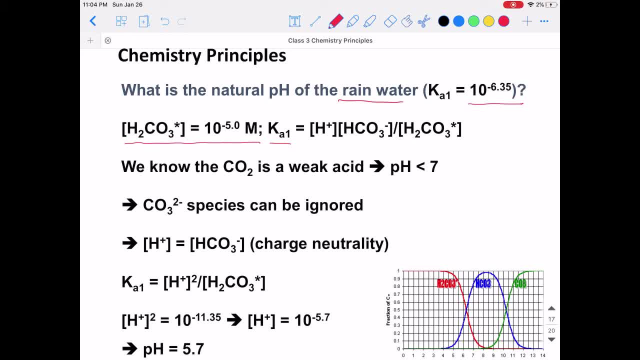 multiplied by the concentration of the bicarbonate ion, divided by the concentration of the carbonic acid. OK, So further, because of the, so, as we have shown here, because the carbon dioxide is a weak acid, the pH is going to be less than 7.. 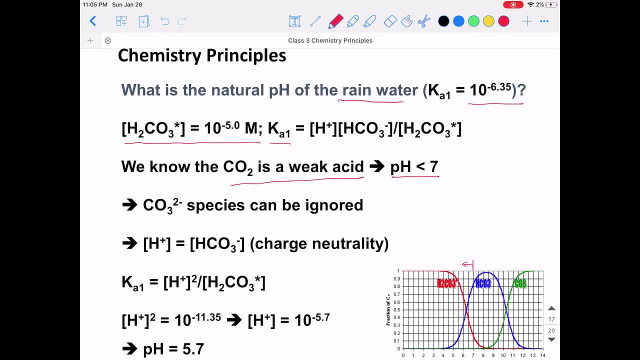 Again, I'm going to draw it here. So we're not going to have any carbonate ions in the solution Right. So under this situation the carbonate species can be ignored. So because of the charge neutrality, the proton concentration is going to be equal. 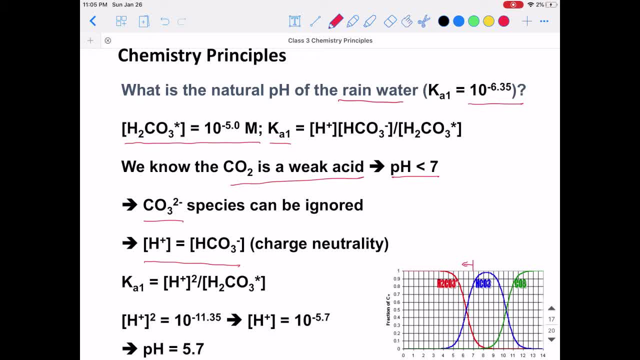 to the bicarbonate ions. So these two concentrations are the same. So then we can plug in the concentration of the bicarbonate ion. So we're going to have the square of the proton concentration divided by the carbonic acid concentration equal to 10, to the negative 6.35.. 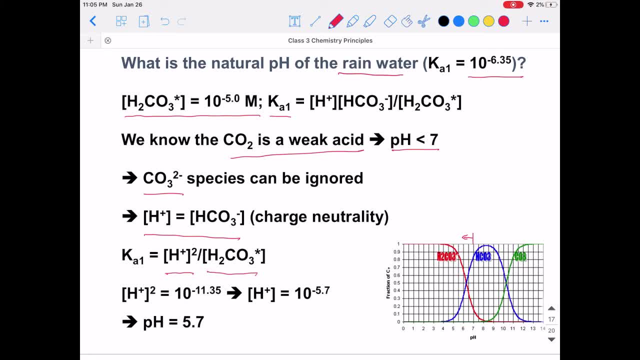 Right, So further, we have the concentration of the carbonic acid coming from here, So we can calculate what is the concentration for the protons And based on the definition of pH, we're going to take the log 10, right of 10 to the negative 5.7.. 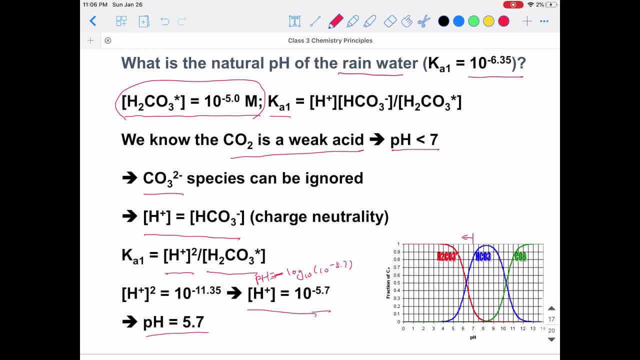 And also remember the negative sign here. So the pH is equal to 5.7.. You can see that for the natural rainwater it's going to be under an acidic condition, Right? So also we can see from this: 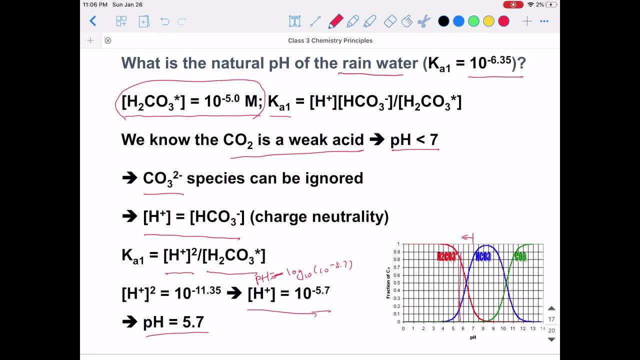 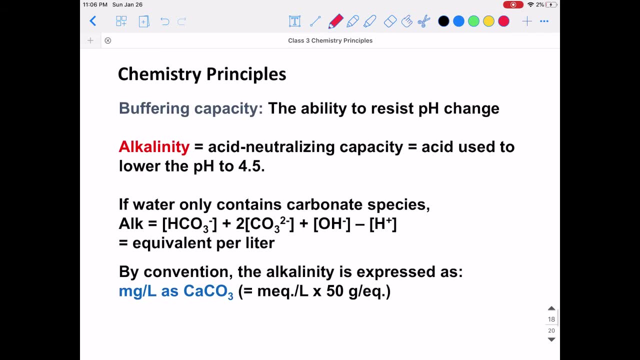 This graph here. so under a pH of around 5.7, you can see that the concentration of the bicarbonate ion is around a quarter of the carbonic acid concentration Right. So further we have the definition of the buffering capacity. 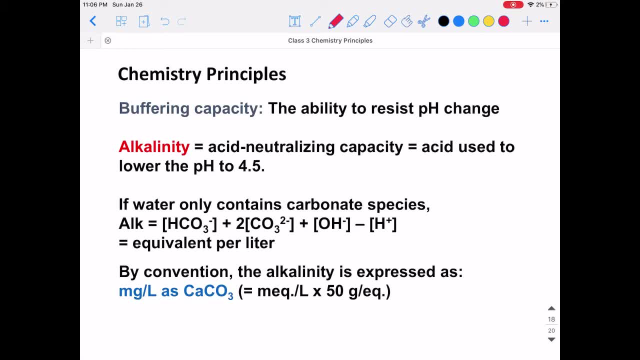 So the buffering capacity is defined as the ability to resist the pH change. So to represent this capacity, we need to define a new A term or define a new parameter called the alkalinity. So alkalinity is defined or can be calculated based on the coming. 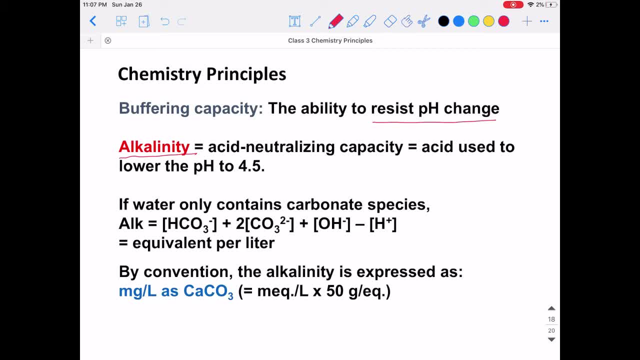 from the acid neutralizing capacity. So basically that is the acid used to lower the pH to 4.5.. OK, So for the water system that only contains the carbonate species, then the alkalinity can be calculated by the concentration. So this is the concentration of bicarbonate ion. 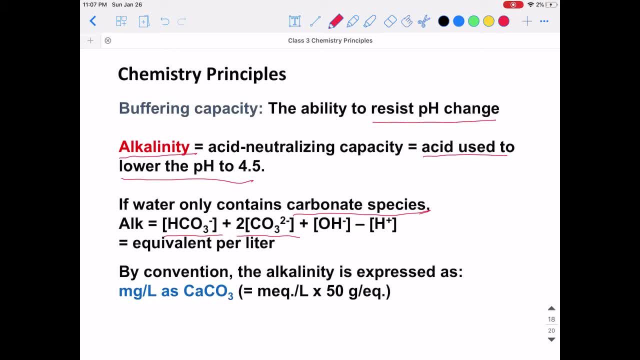 plus twice of the carbon ion, Because the carbon ion needs two protons to neutralize these species, Right. And then we also need to consider the concentration of the hydroxyl ion, Right, And also we need to minus the concentration of the proton ions. 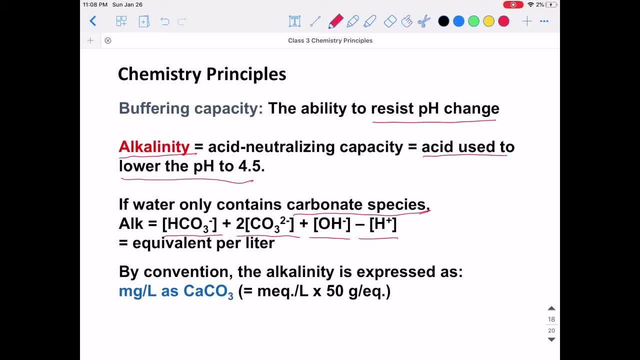 And also the alkalinity is shown In the unit of equivalent per liter. So basically, by convention the alkalinity is expressed as the milligram per liter as calcium carbonate. So basically we want to use the equivalent weight of calcium carbonate too. 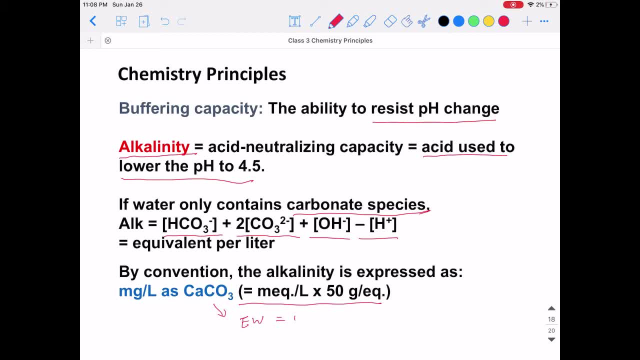 And we have already calculated that the equivalent weight of calcium carbonate is 50 grams, Right, 50 grams per equivalent weight, Right. So basically we want to use the equivalent weight of calcium carbonate. So basically, what we can do is we can first calculate. 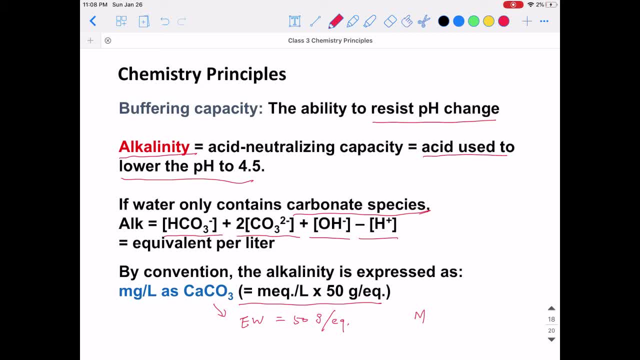 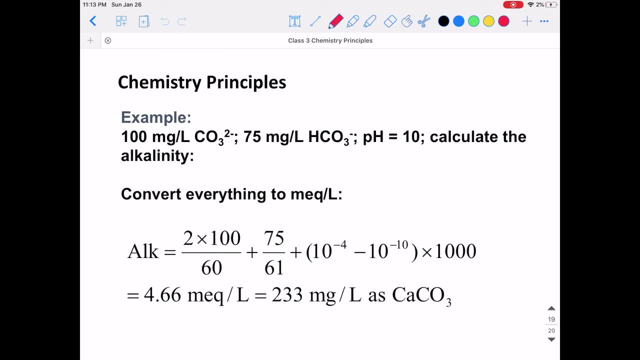 the molarity of all of these acid neutralizing species And then just multiply that by the equivalent weight And then that is going to give us the alkalinity. So let's work on our final example here. So it wants us to calculate what is. 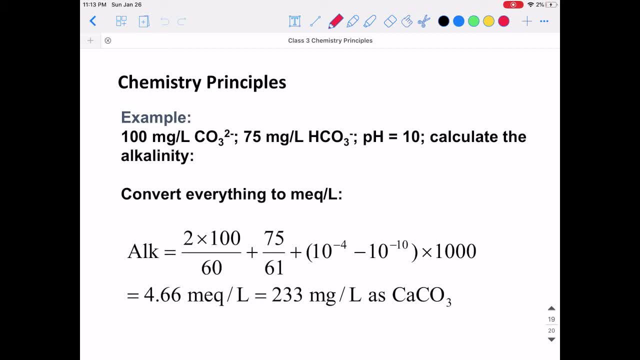 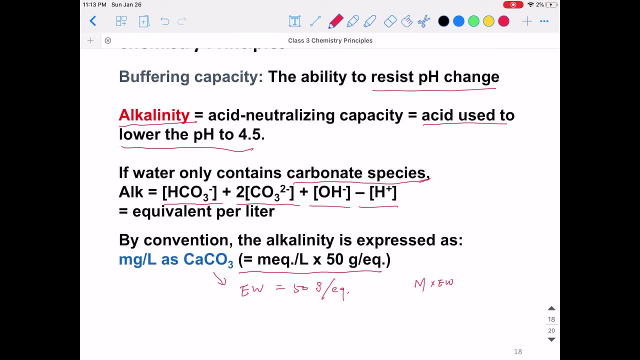 the alkalinity of a solution that's containing 100 milligrams per liter of the calcium carbonate, 75 milligrams per liter of bicarbonate ion under a pH of 10.. Right, So according to the equation here for calculating the alkalinity, 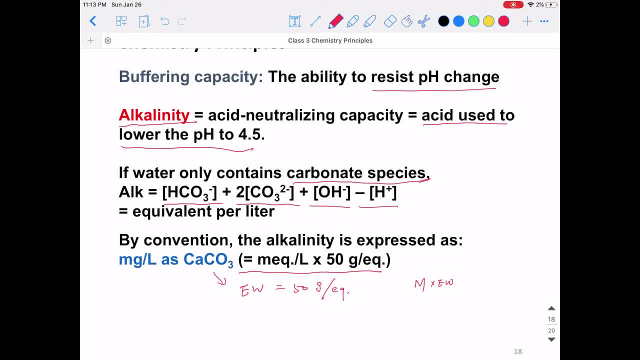 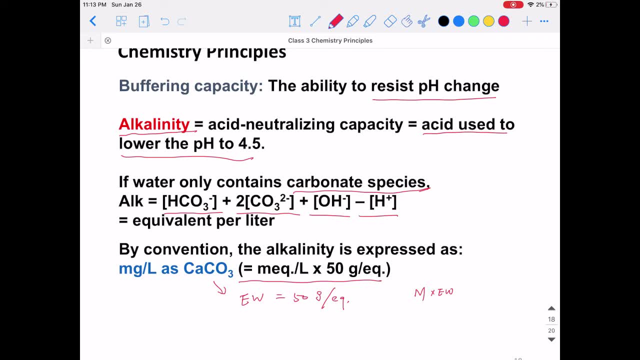 So we need to first calculate what is the molarity of all of these species that can neutralize the protons Right. So we need to notice that we have to multiply 2 in front of the carbonate ions, because one carbon ion can neutralize two protons. 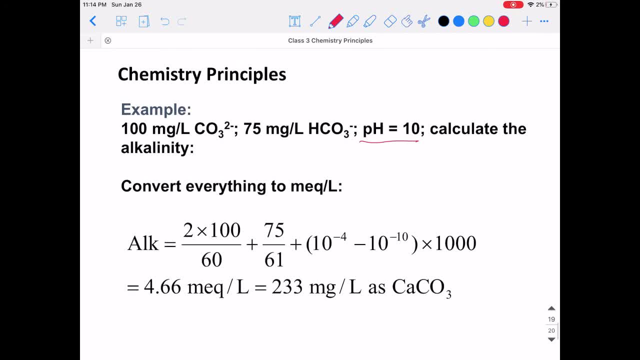 Right, So we need to notice that we have to multiply 2 in front of the carbon ions, because one carbon ion can neutralize two protons. Right, So then we can directly use the condition here, Because we already know the mass concentration of the bicarbonate ion. 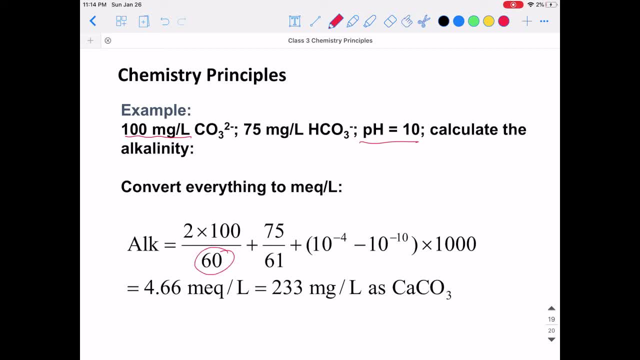 We can directly divide that by the molecular weight of the bicarbonate ion, which is 60. And then we need to remember that we need to multiply 2 in front of this mass concentration For the bicarbonate ion. we can divide 75 by 61,, which is the molecular weight of the bicarbonate ion. 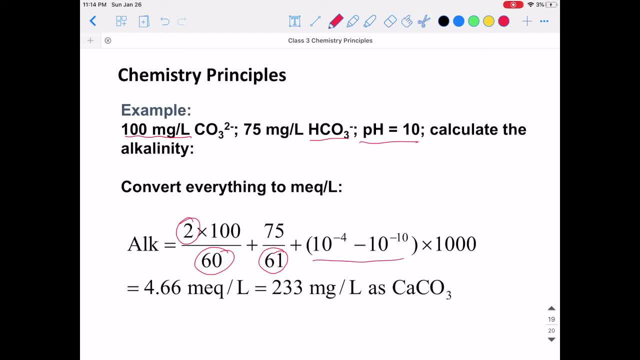 And also we need to consider the concentration of the hydroxide ion and also the protons right. So under a pH of 10, then the hydroxide ion concentration is going to be 10 to the negative 4.. And the concentration for the proton is going to be 10 to the negative 10.. 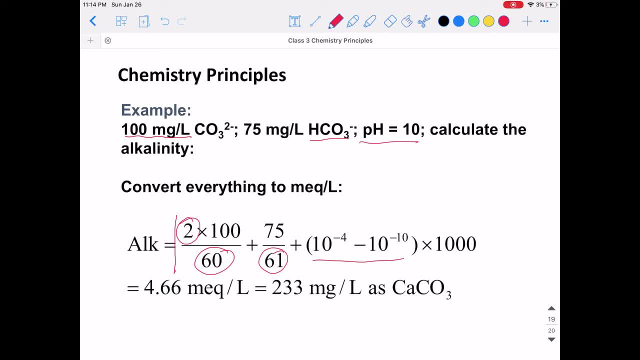 So also one thing we need to notice is that here to calculate the concentration of the proton that can be neutralized, we were using the unit of milligram per liter, right? So we're calculating basically the milliequivalents per liter. 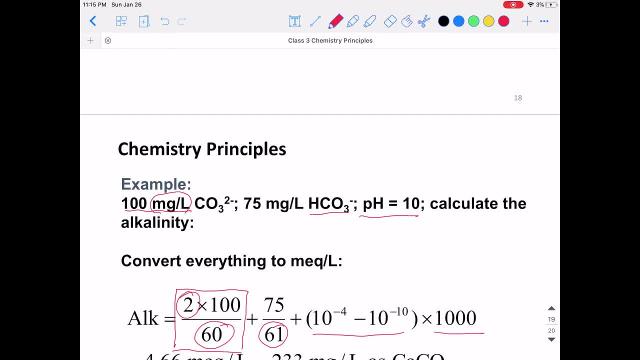 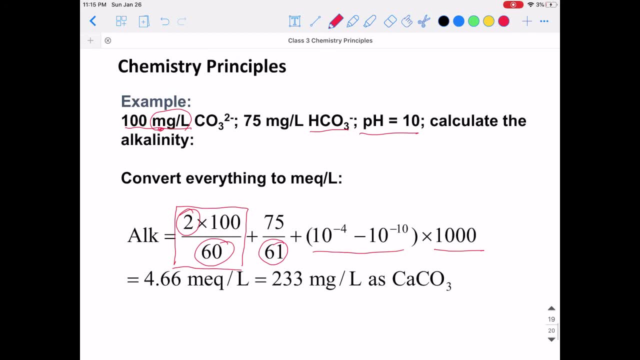 So under this situation we also need to multiply the concentration of the hydroxide ions by 1,000, because here we didn't convert that into gram per liters. So this is going to give us 4.66 milliequivalent per liter, right. 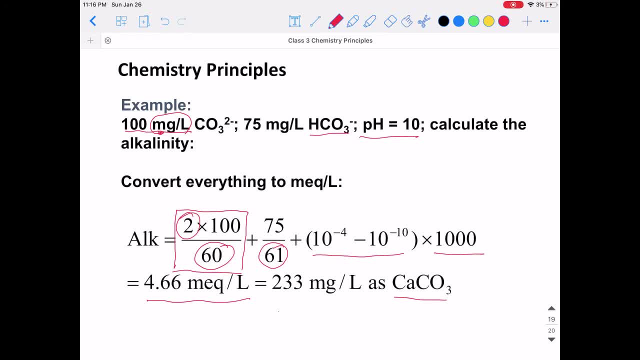 And finally, we need to multiply. We need to multiply the equivalent weight of the calcium carbonate, which is 50 gram per equivalent right, And multiply this number by 4.66, and that's going to give us 233 milligram per liter as calcium carbonate. okay, 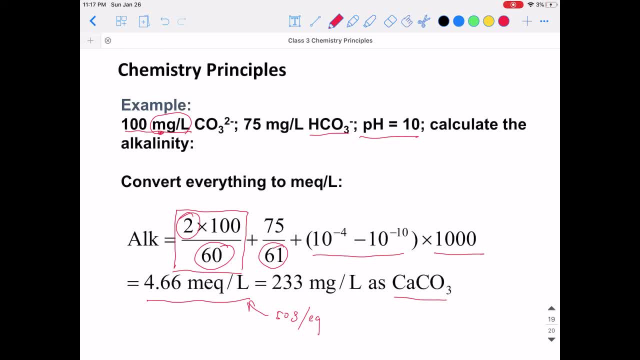 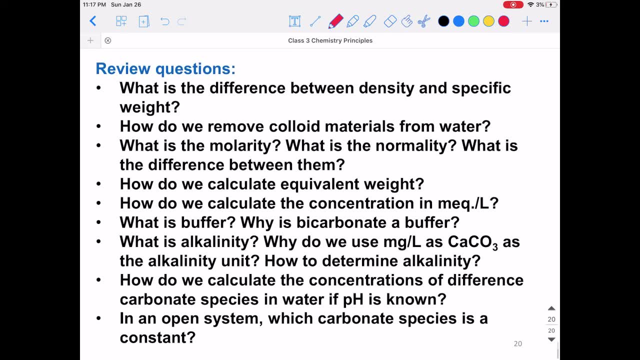 So I hope that this example is clear enough so we can use that to calculate what is alkalinity for certain species of solution, right? So now let's review the questions we have gone through in this class. So what is the difference between the density and specific weight, right? 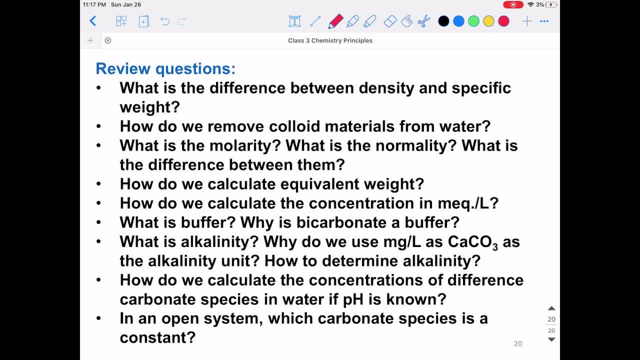 So for the density it's just based on the mass of the species, right, And that mass and the volume of the species and specific weight is in terms of the water. okay, So also we want to understand how do we remove the colloidal materials from the water? 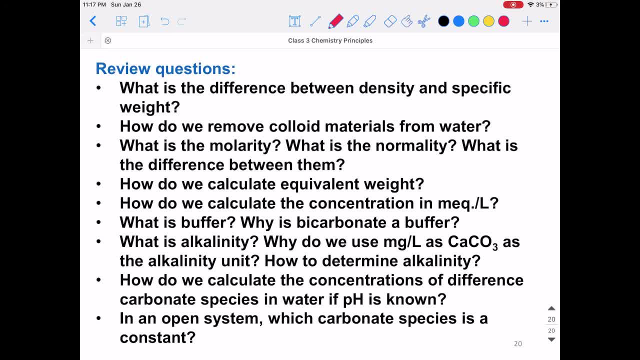 We can use filtration, right. We can also use ultracentrifugation, right. What is the molarity and what is normality? So normality is dependent on the transfer of the electrons or the protons. What is the difference between them?